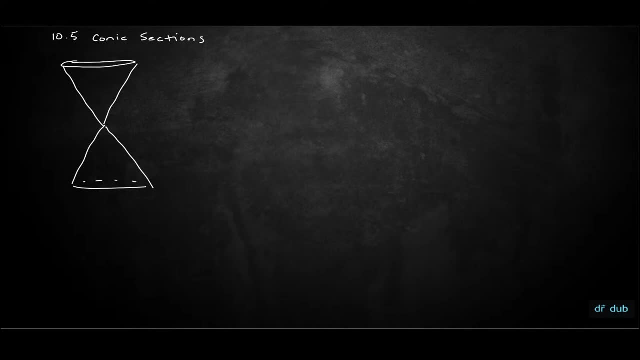 L In order to create a, an ellipse L, And you'll be able to see that it looks like this: L L Okay, 10.5 conic sections: L. Here's the shape: L L. 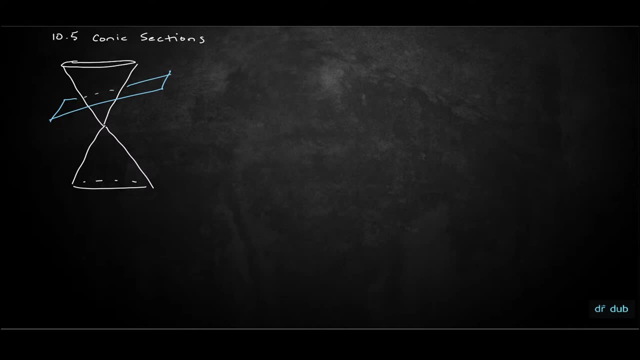 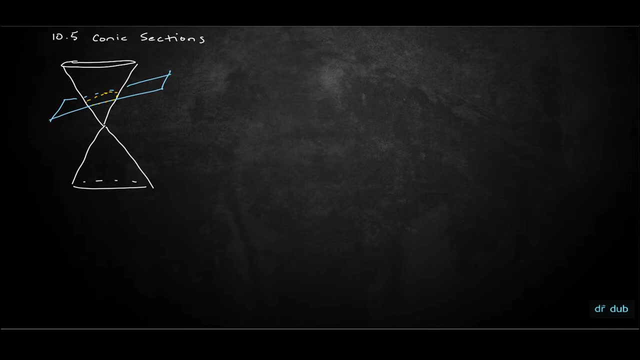 would get an ellipse if you had a vertical plane, maybe something like this, where we get hyperbola. so you cut through this cone or these- it's really one cone, even though it has two pieces- a top part and a bottom part- and you cut through this cone and you cut through this cone and you cut through this. 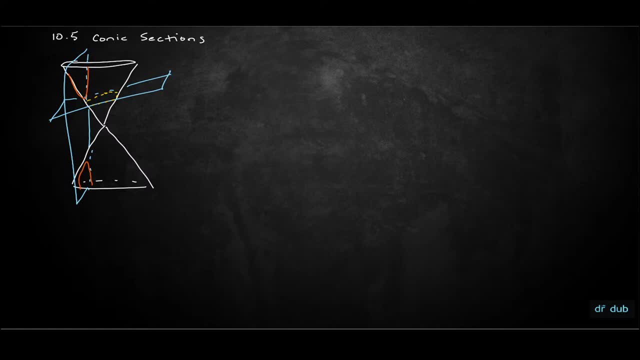 and if you cut through the cone at different angles, you get different shapes, and if you cut just the right angle, you get a parabola. so between the angles that give you ellipses and the angles that give you hyperbolas, you'll get parabolas. and depending on which cone 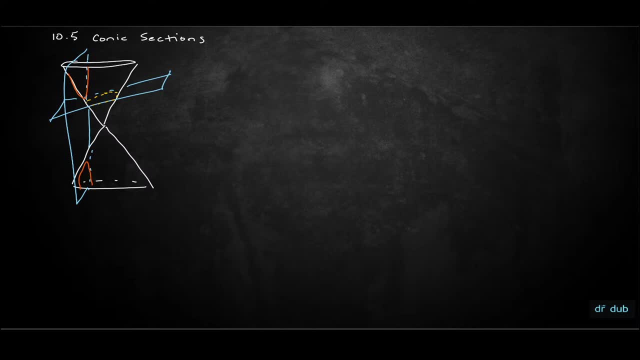 you have. you have a shorter cone or, sorry, a steeper cone versus a less steep cone. you get different parabolas, different ellipses and things like that, but that's kind of the idea. these are called conic sections or conic cross sections, depending on how you cut through the cone. so the first thing i want to do is 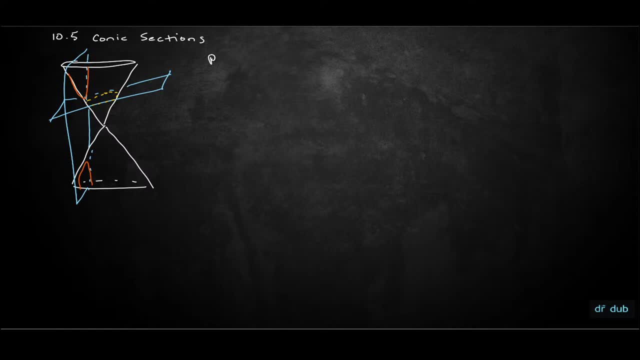 talk about parabolas. so parabolas, parabolas are conic sections and the definition of a parabola. i'm going to give a geometric definition and then derive the equation of the parabola from that geometric definition. so a parabola. 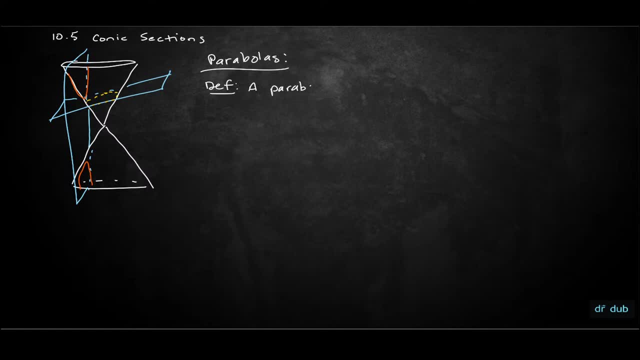 a parabola is the set of all points in a plane that are equidistant and, and the set of points that are equidistant from a fixed point p, called the focus. equidistant from a fix fixed point p: equal distance from a fixed point p. 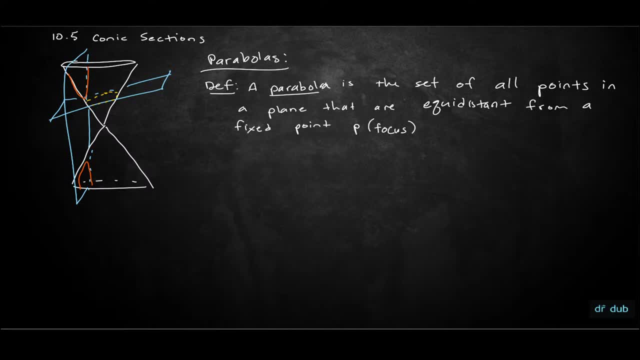 distance from a fixed point, p, and a fixed line called the directrix, And it tells you the direction of the parabola. So let me draw a graph of this parabola. I'll just draw it going through the origin right here. 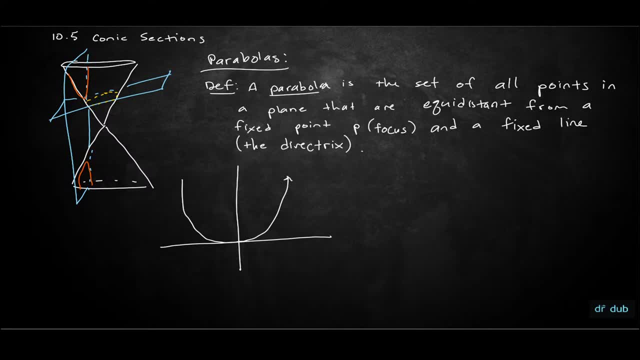 So this is a parabola. I just happen to have it go into the origin. It doesn't have to, but the derivation here will be a little easier If you're going to draw a graph of this parabola. I don't know if it does. 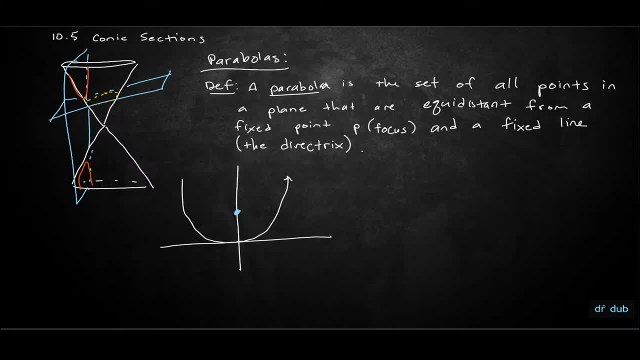 So let's say this is a point P, It's called the focus. We'll say it's at the point 0P, And then the directrix is this line: right here, Y equals negative P, And every point on this parabola should be the same distance. 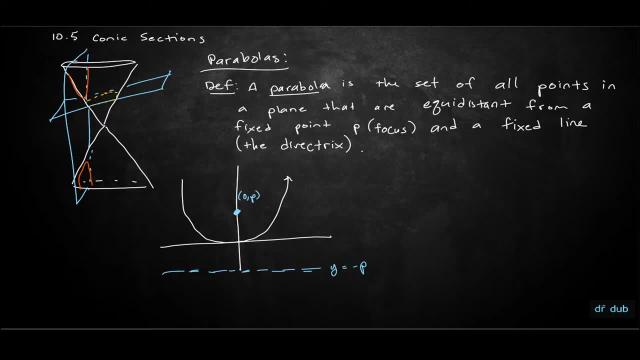 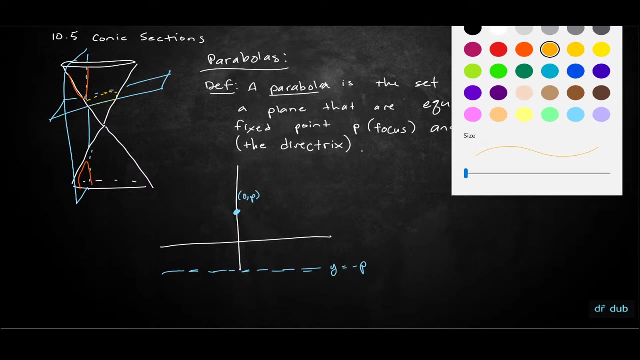 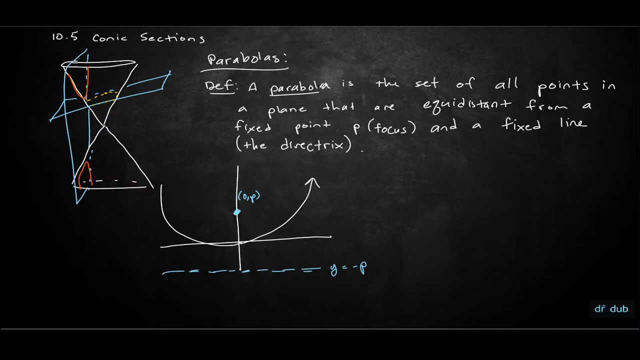 from the focus As the directrix. So actually this parabola needs to be a little bit more wide, Kind of like this: So this distance here should be the same as this distance here, So these two lines are the same distance for any point on the parabola. 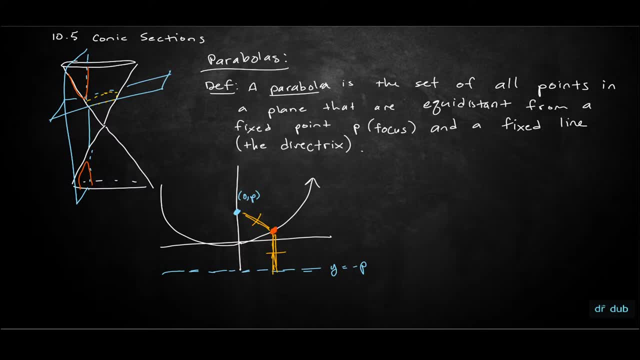 We'll call it a point XY. So parabola is the set of all points XY in the plane that are equidistant from a fixed point P called the focus. So your focus is right here in blue, So equidistant from a fixed point P. 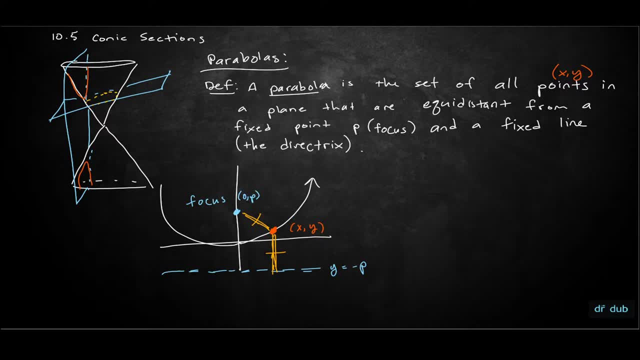 which is the focus and the fixed line called the directrix. So this is the directrix, And think about this point right here at 0, 0.. This point, right here at 0, 0, is a distance of P, So this would also be a distance of P. 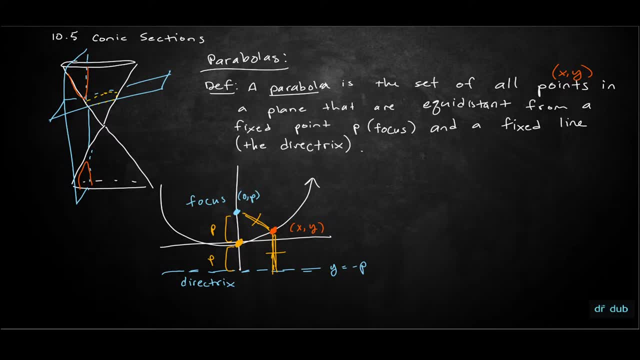 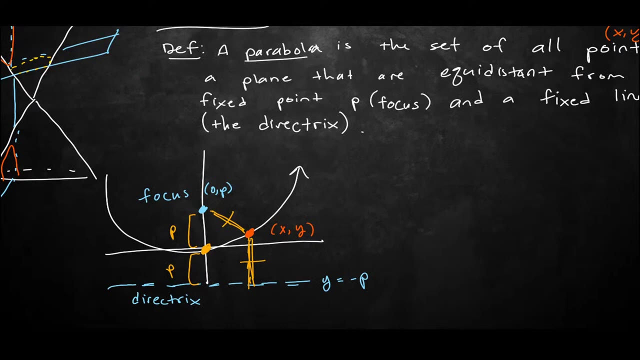 So that's how we know that that directrix is at Y equals negative P. All right, So let's derive the equation of a parabola, knowing all of this information now. So, oops, goodness, just zoomed in somehow. 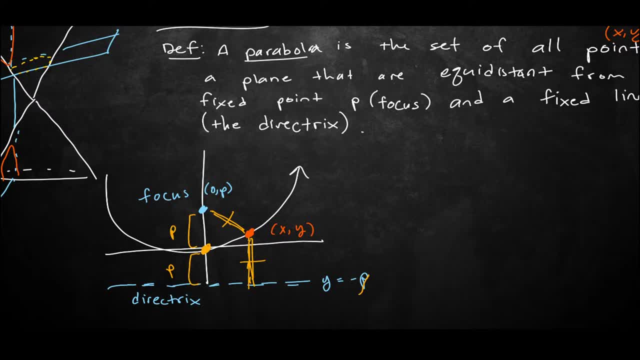 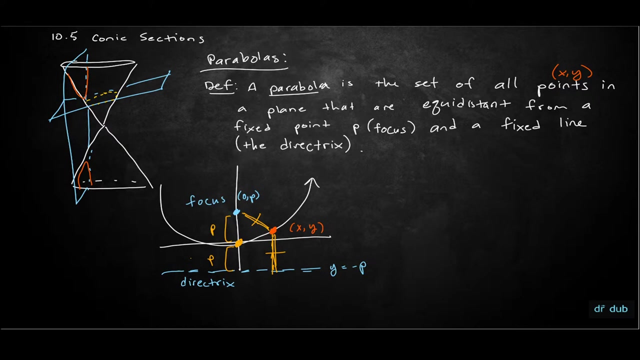 Let me zoom out. OK, So now, how do we get the equation of the parabola? OK, So now, what we're going to do is we're. so. what is the equation of the parabola? let's see. is it lagging? let me see. 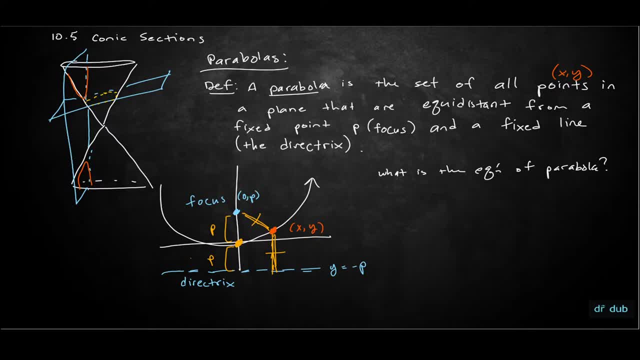 i'm not sure what's going on with the uh visuals. i'm not sure. i have to check on that uh later. it's weird. uh, try to keep going and see if it'll uh maybe work itself out. it's weird, okay, um, let's see what is the equation of the parabola. 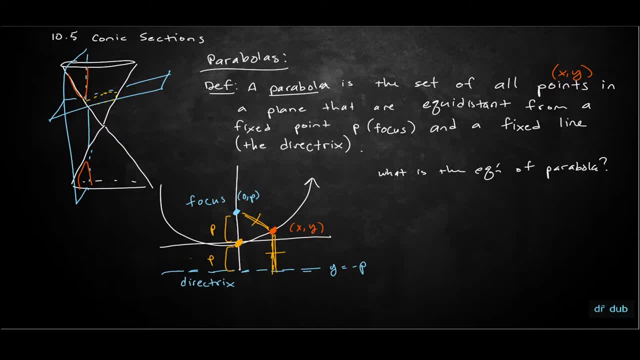 well, what do we know? we know that the distance between these two points, the focus and x y, should be the same as the distance between x? y and the line. so find the distance between the first two points, the focus and x y. so the distance d1. 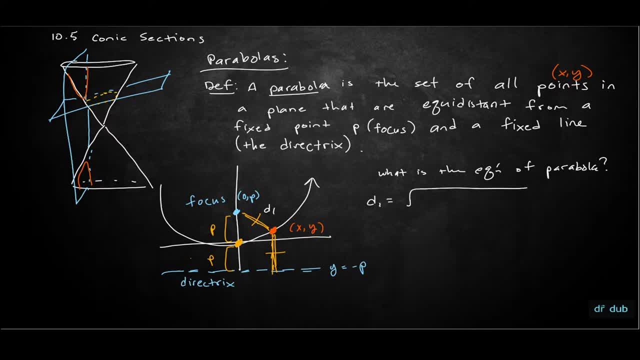 would be square root x minus 0 squared plus y minus p squared, and distance d2 be the square root of x minus x squared plus y minus negative p squared, and those should be the same distance. so then we equate those two, so d1 equals d2 by definition of the parabola. 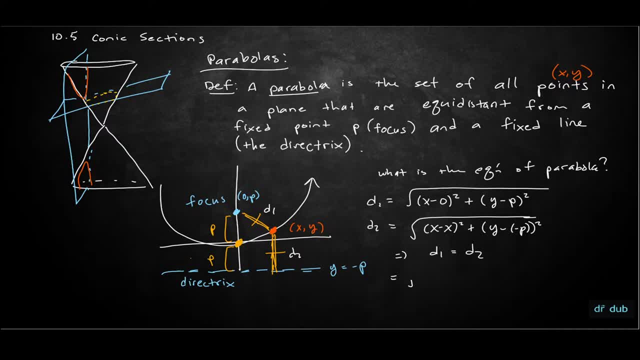 and that would tell me square roots of x squared plus y minus p squared should be equal to square roots of y plus p squared. so now square both sides. i get x squared plus y minus p square equals y plus p. whoops, y plus p square. so 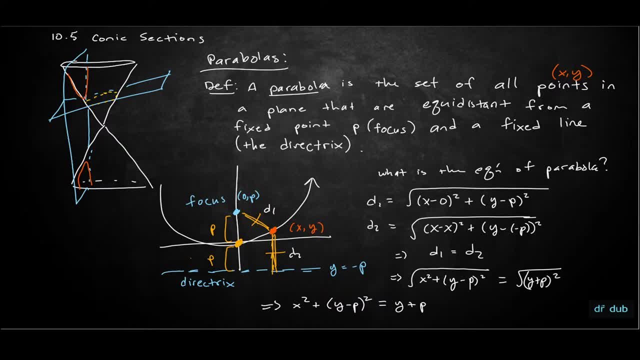 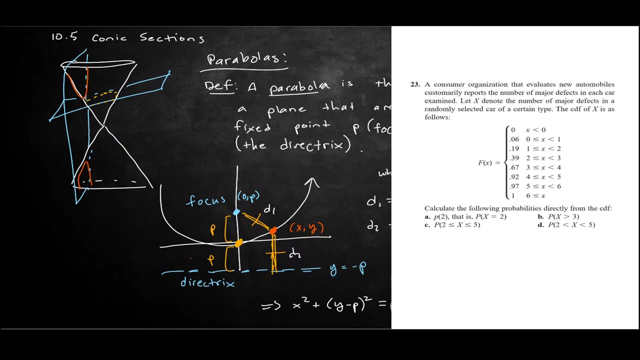 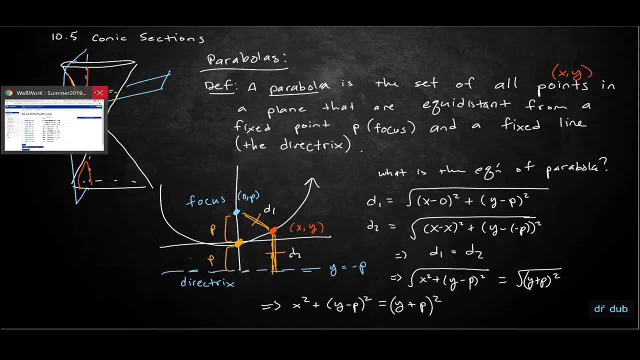 okay, you get x squared plus y minus p squared equals y plus p, And so let me see, I wonder if maybe it's I just have too many applications open. let me see if that helps. Now let's do some algebra to simplify. 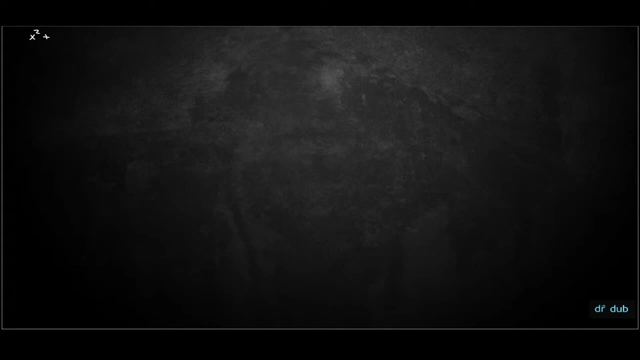 So that'll give us x squared plus y squared. Okay, Minus 2yp plus p squared equals y squared plus 2yp plus p squared, Just by squaring out both sides. Let me see if that helped a little bit. Yeah, that seems to have helped a little bit. 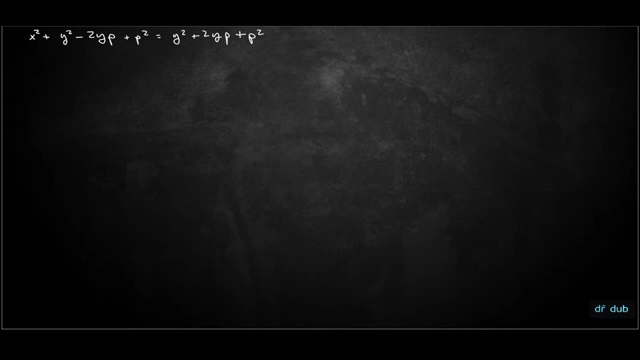 Too many applications open. Okay, Let's see Some algebra now. just cancel some stuff on both sides. This y squared can go away. this p squared can go away. I can move this over to the right-hand side just to simplify a little bit. 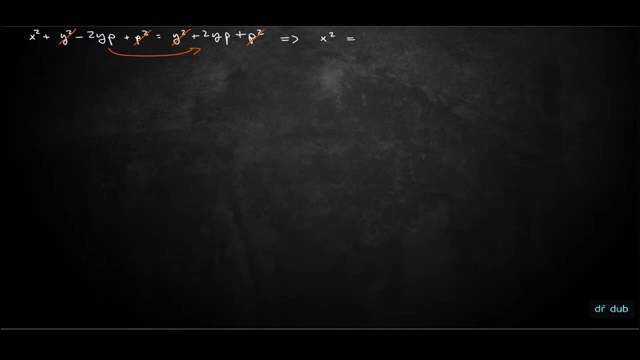 And we get x squared. x squared equals 4yp, And so y is equal to 1 over 4p x squared. And if we let a equal 1 over 4p, then we get y equals ax squared. Okay. 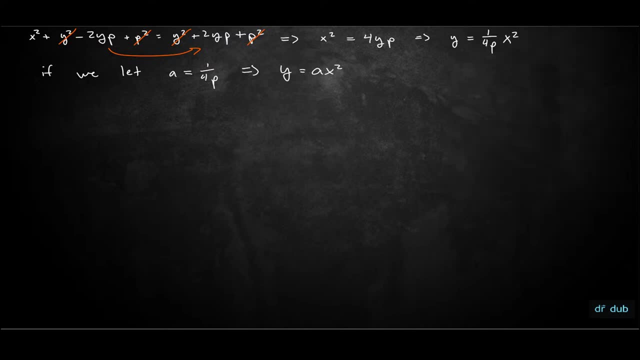 Which we know is a very basic form of the parabola, But now we know there's more to it than just y equals ax squared Passing through the origin. there's also a focus and a directrix tied up in that coefficient a. 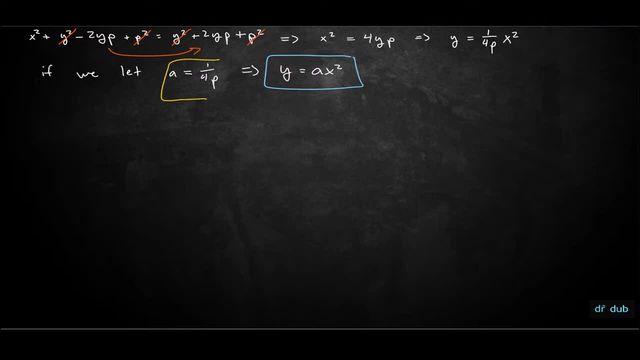 So just note here this is important: a is equal to 1 over 4p And little p is the distance from the vertex, From the vertex to the focus. So little p is the distance from the vertex to the focus. 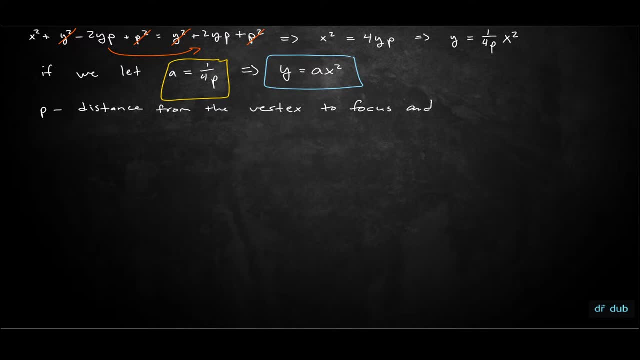 And from the vertex to the directrix. Now let's floating. Well, if a is greater than 0, opens up. Yes, a is less than 0, opens down. If a is greater than 0, opens down. Well, totallyfecture this and all of these Father. 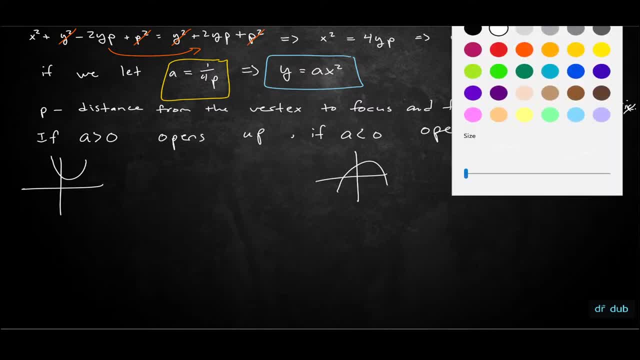 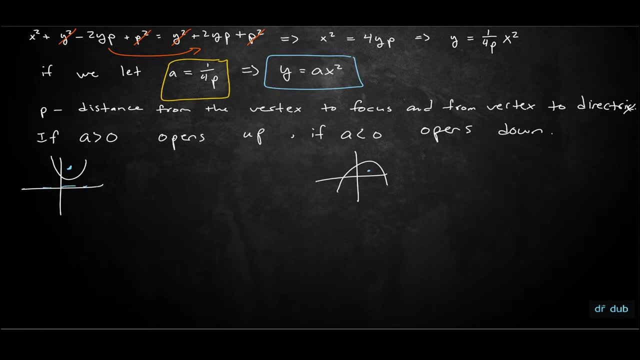 so you don't have to worry quite so much and get free in terms of this matrix and in each case we'll we have a focus and a directrix. however, we could also have X as a function of Y, so, similarly, we're not going to derive it, but 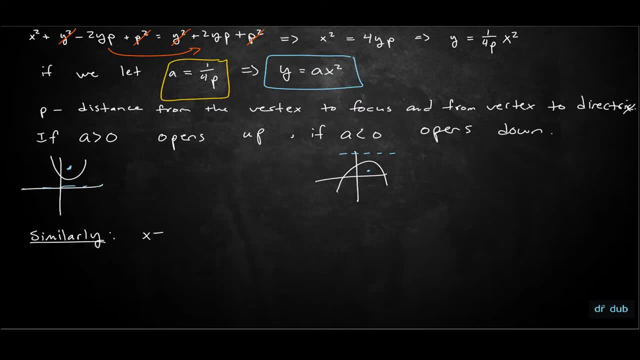 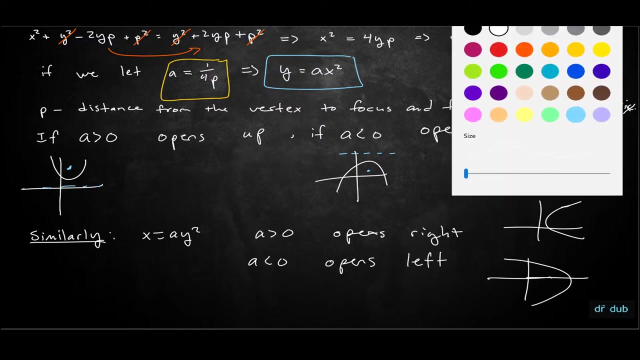 similarly, we could have X equals a y squared, and if a is greater than zero, it opens to the right, and if a is less than zero, it opens to the left. so we could have parabolas on their sides as well, with the focus and a directrix. 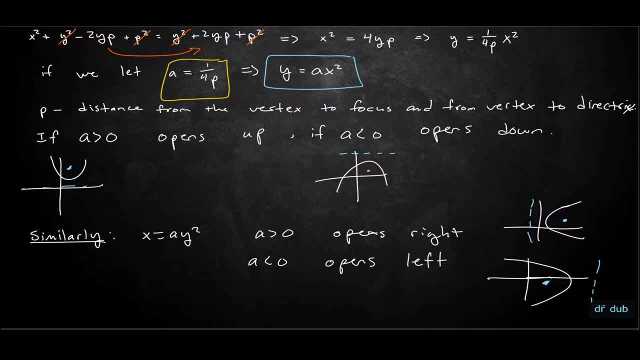 you. so in each case that coefficient a is equal to 1 over 4 P and P is the distance from the vertex to the directrix. so let me just highlight that distance P right here. so let me just highlight that distance P right here in each case. 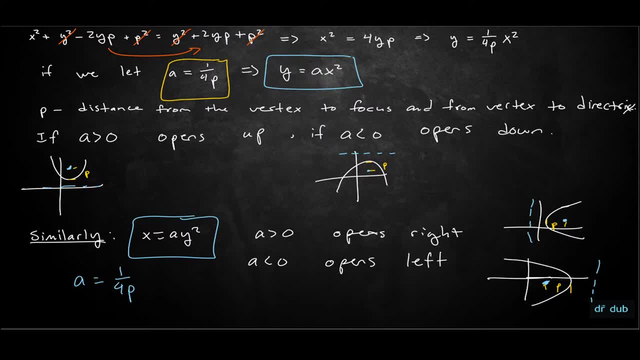 so yeah, that's uh, that's pretty much it for parabolas. I mean, of course we can. so yeah, that's uh, that's pretty much it for parabolas. I mean, of course we can them left to right up, down all that stuff. but these basic equations I'll 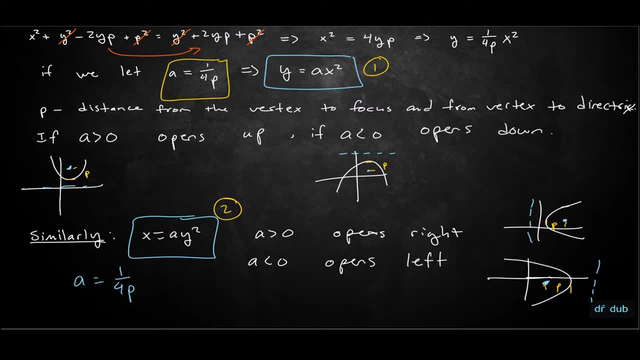 call them 1 & 2. those are for the unshifted parabolas at the origin, but from there you could shift it left, right up down all that stuff. so any questions about the derivation? we'll do some examples now if there are no questions. 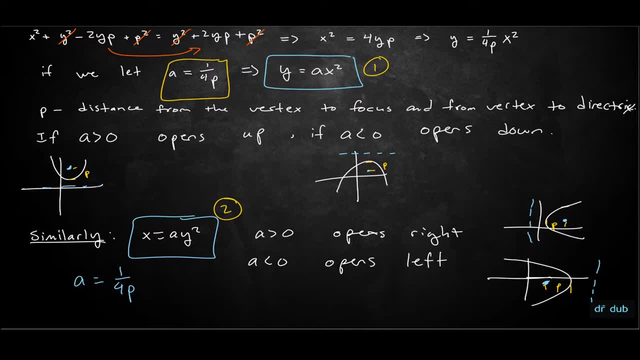 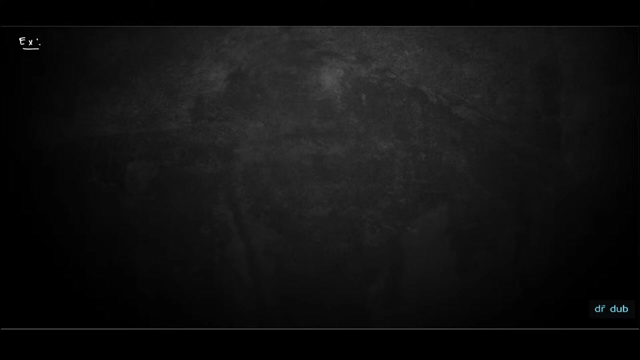 you okay. first example: it says: find the equation. so find the equation. it should say P, equation of the parabola in the form y: x equals f of y, so x equals f of y if the focus is at the point negative, two, zero and the directrix. 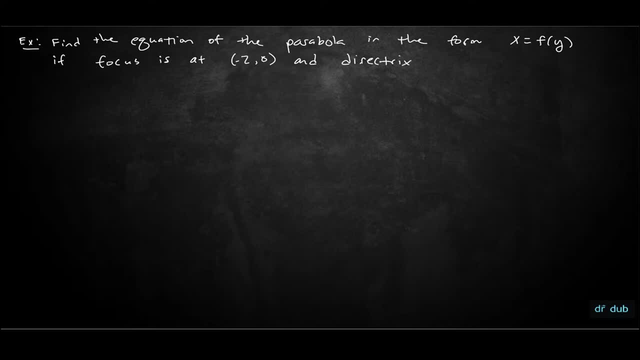 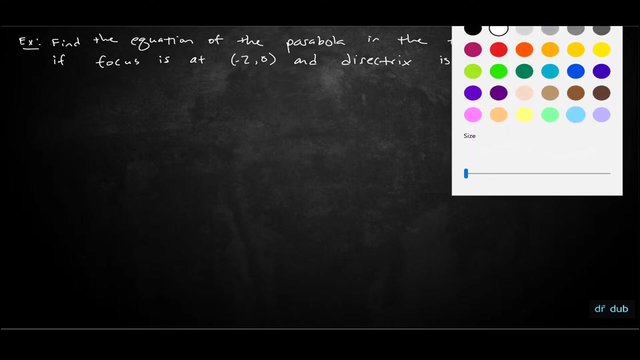 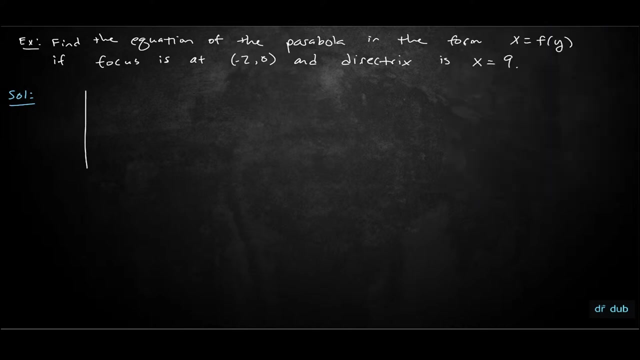 is, the line x equals nine. so we've got a problem parabola. let's try to figure out what it looks like first, and that'll help us kind of solve the problem overall. so let's look at the parabola. just draw some axes here so we know that there is a directrix. 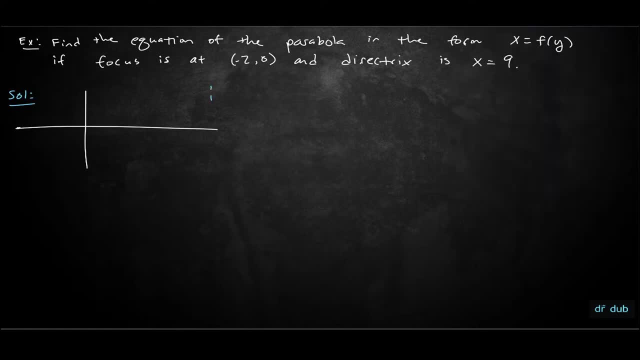 at x equals nine. so that's like over here at nine, and we know there's a focus at negative two and that's like right here: negative two, 2, 0.. So what do I know? I know that the vertex needs to be exactly halfway. 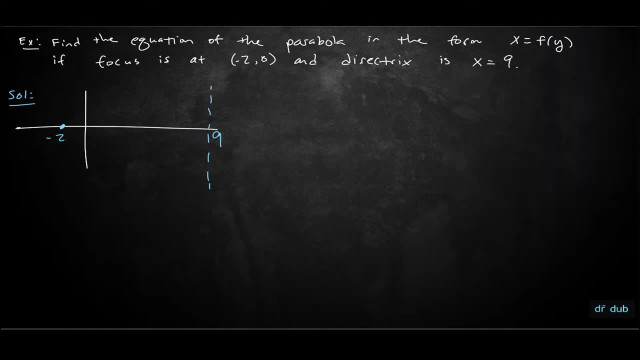 between those two, and so the vertex should be somewhere here and it should open up away from the directrix. So it's opening to the left this way, probably a little too steep there, So something like that. But what is the vertex? So the vertex is halfway between: 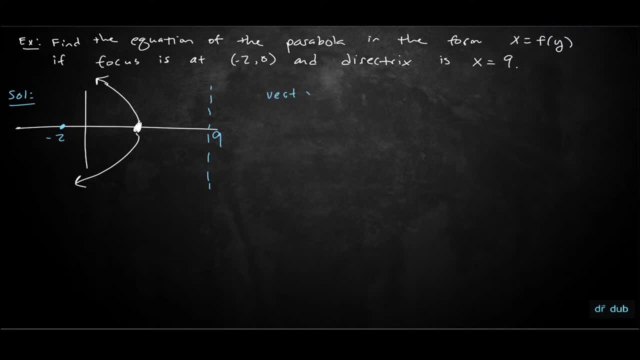 the focus and the directrix. So the vertex is halfway between the focus and the directrix. So we know the y-value is going to be 0, but what's halfway between these two points? So x-bar, the midpoint, midpoint x-bar, is going to be negative, 2 plus 9 over 2,. 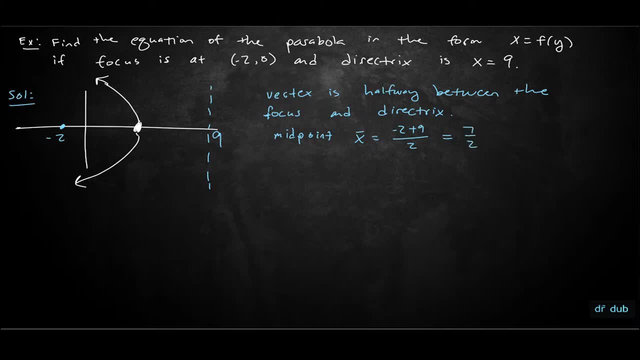 which is 7 over 2.. So this x-value is 7 over 2.. So the vertex is at 7 over 2, 0.. It has to be the same vertical line. y equals 0, but the x-value is halfway between and the 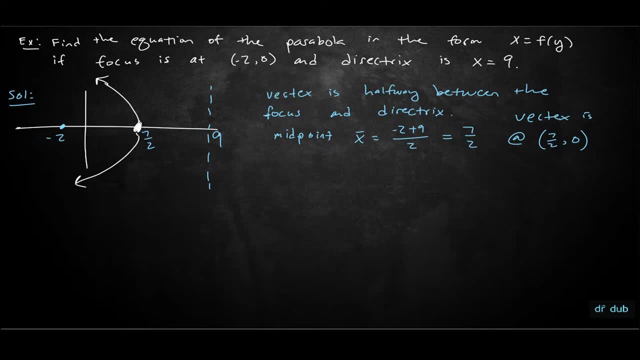 midpoint between two values is the 7 over 2.. So the vertex is at 7 over 2, 0.. So the x-value is halfway between, and the midpoint between two values is the sum divided by 2, or the average value. 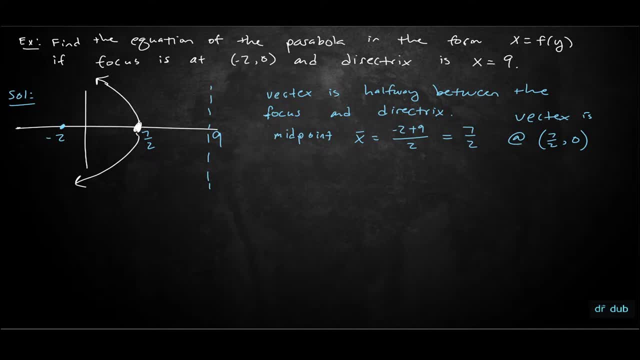 So that's the vertex, So I got the vertex, but I also need the coefficient. So let's see, I know, let's see, I'm shifting to the right my x-value by 7 over 2.. So x minus 7 over 2 should be equal to a times y squared. 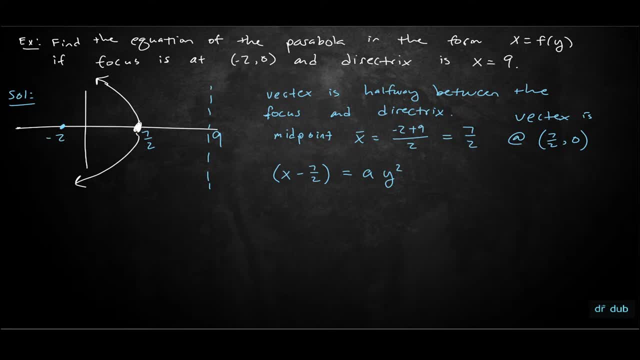 Because I'm not shifting y at all. So y is shifted by 0,. x is shifted by 7 over 2 to the right. So I do x minus 7 over 2.. Now a is equal to 1 over 4 p. 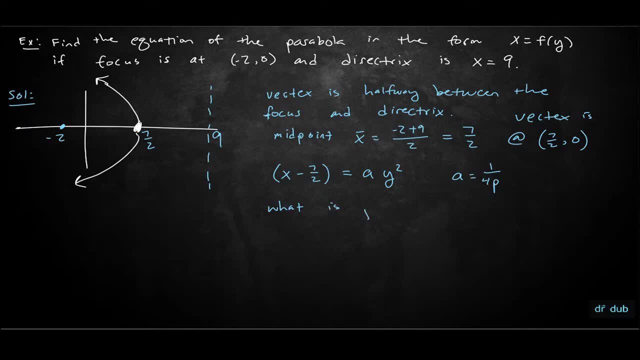 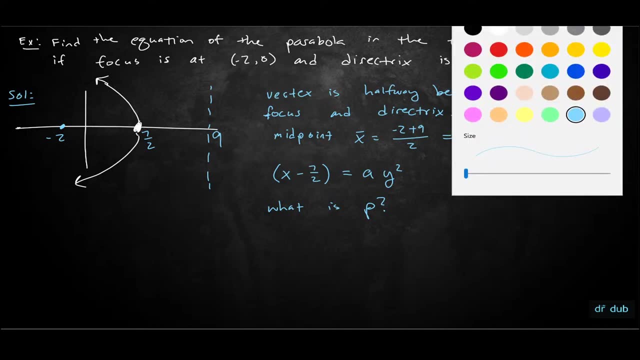 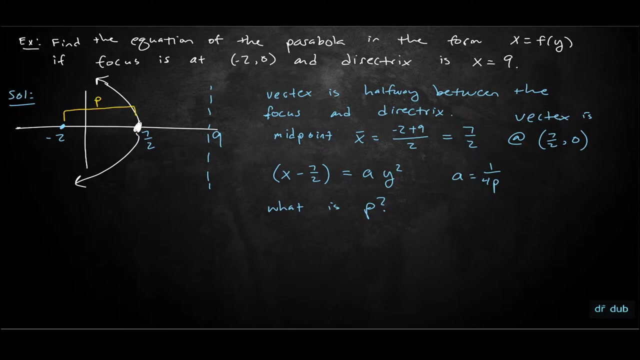 And what is p? So what is p? Well, p is the distance between the vertex and the focus. So what is that distance right there? So p is going to equal 7 over 2 minus negative 2, which is 7 over 2 plus 2.. 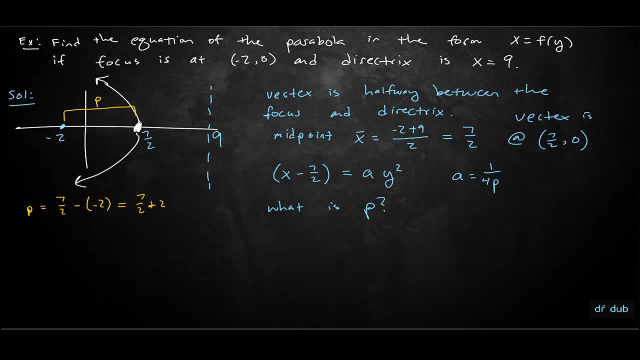 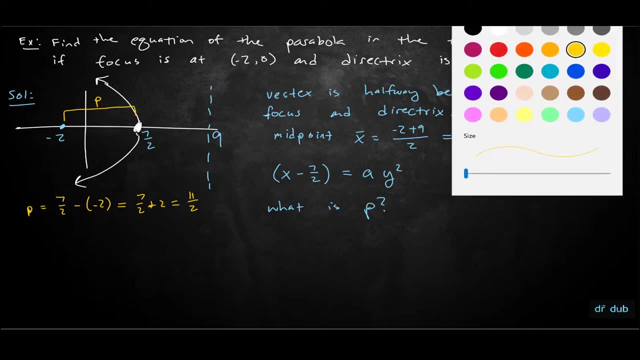 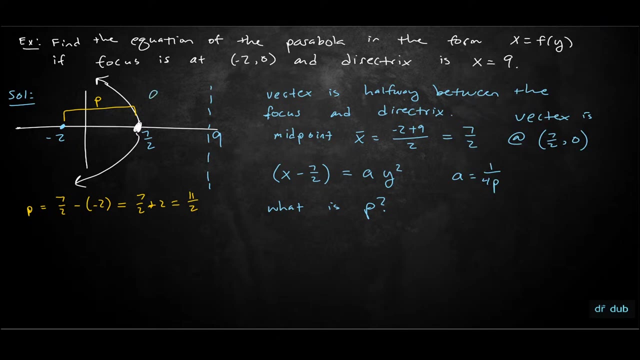 Which is going to be 11 over 2.. So little p is 11 over 2. Or at least absolutely So. it opens to the left, though. so we know a is negative, so a is less than 0. So a is going to equal negative 1 over 4 times 11 over 2.. 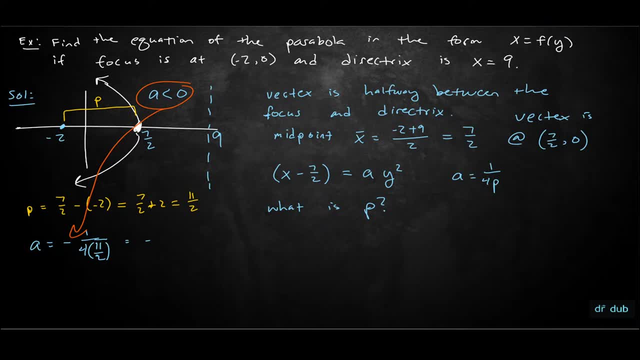 So this is going to be negative 1 over 22.. So that's what a is And we plug that in. so we get x minus 7 over 2 equals negative 1 over 22 y squared. And we can solve for x and say that's going to be negative 1 over 22 y squared plus 7. 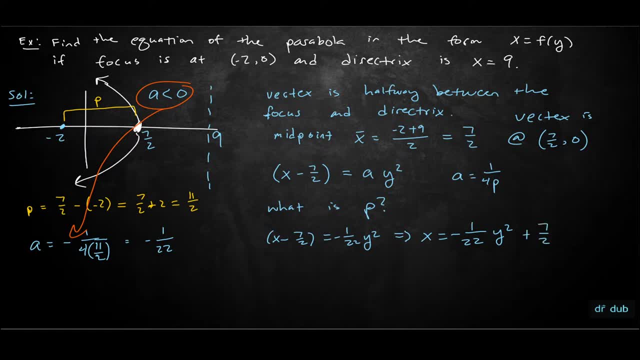 over 2.. And that would be the equation of this parabola. Any questions about that example? Yes, All right, All right, Thank you everyone. Thank you, Bye, Bye, Bye, Bye, Bye, Bye, Bye. 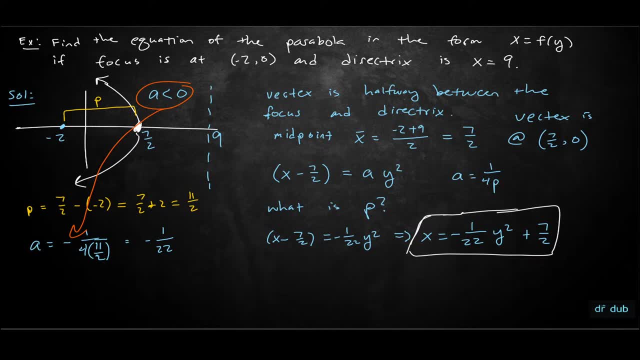 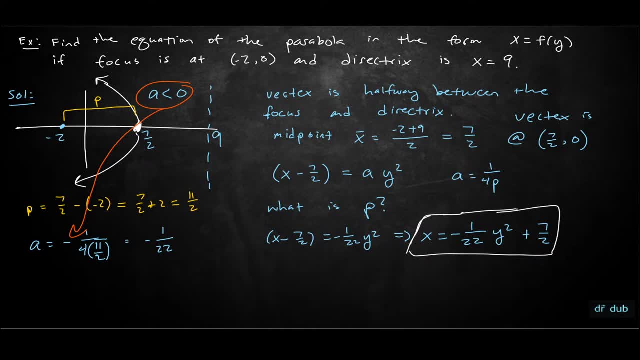 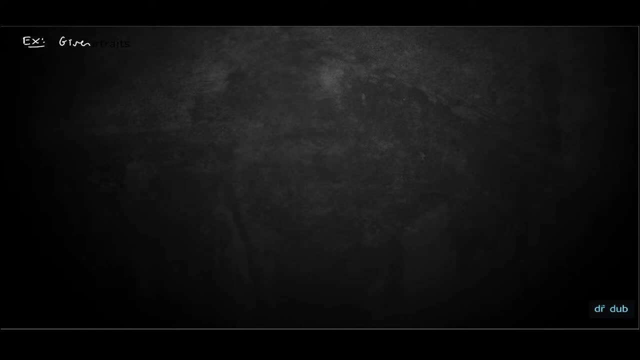 and I want you to find the focus in the directrix. So, example: given y equals 2x squared plus 4x minus 1, find the focus, vertex and directrix and sketch the graph. So find the vertex, focus and directrix of this quadratic, The vertex you can do. 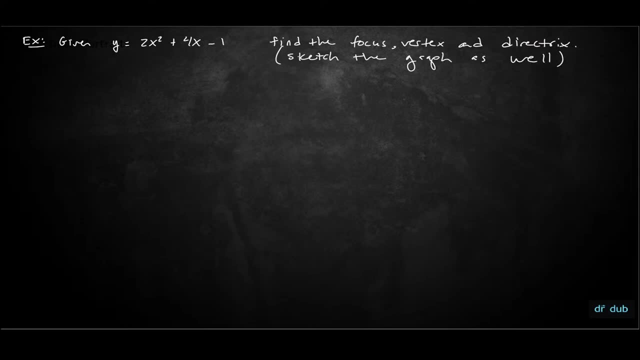 from precalculus Now to big two. Same thing with now the coefficient a, we know, contains the information to get the focus. So let's find the vertex first. So find the vertex first, And my recommendation is just to complete the square. So 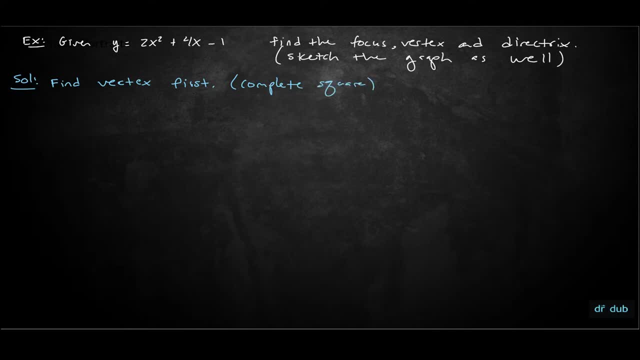 complete the square, And so I'll say that that's going to be: y equals 2 times x squared plus 2x, and then minus 1 goes out here, And to complete that square, divide by 2,, get 1 squared. 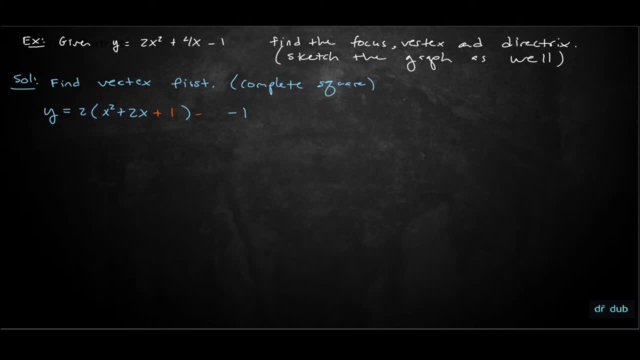 So that and add it, And then minus 1,, actually minus 2, because we're adding 2 technically, since there's a 2 outside of that parentheses. So just highlight that 2 out here. So that's why we have to subtract 2.. So this becomes 2 times x plus. 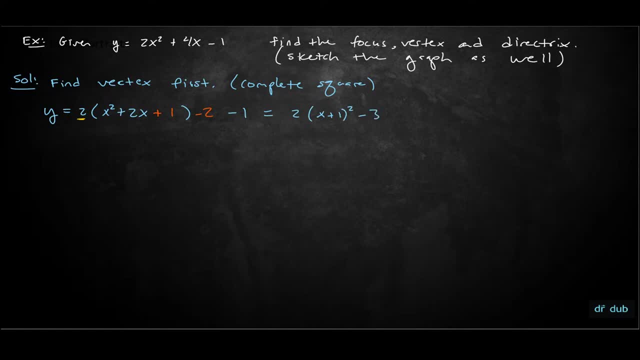 1, quantity squared minus 3.. And so, So now we know the vertex is at: x equals negative 1,, y equals negative 3.. And what do we know as well? We know a is 2, and we know that's 1 over 4p. 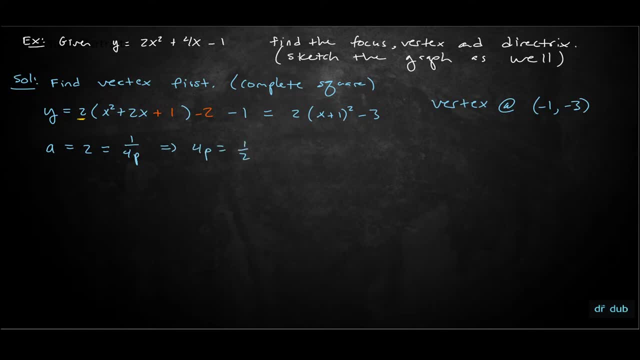 And so 4p should be equal to 1 half, and so p should equal 1 over 8.. So I need to. let's see: is this opening up? It's opening up, so I need to take this vertex and add a y value of 1 over 8.. 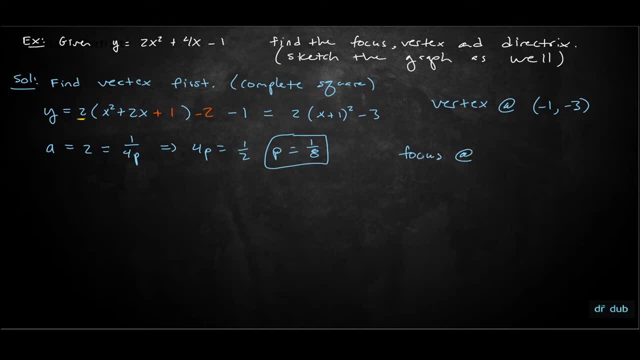 So the focus is going to be at negative 1 comma 3, negative 3 plus 1 over 8.. And the directrix is going to be: y equals negative 3 minus 1 over 8.. And how do I know all this? 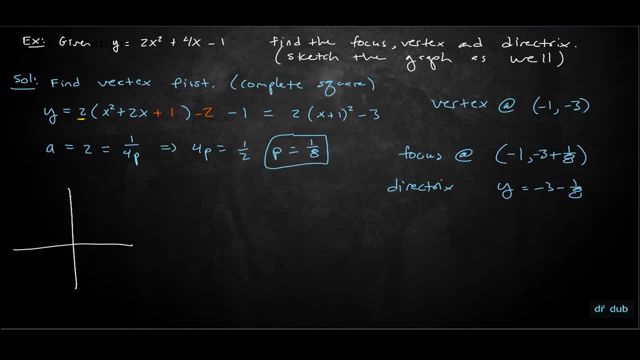 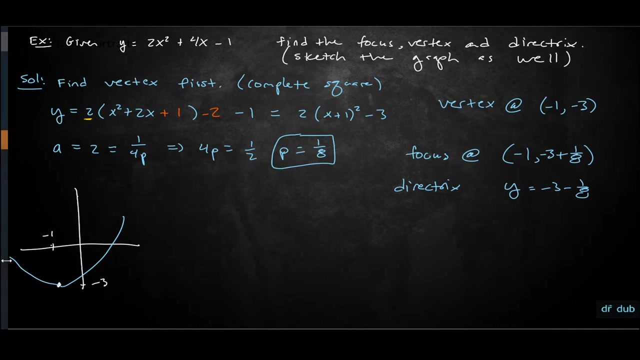 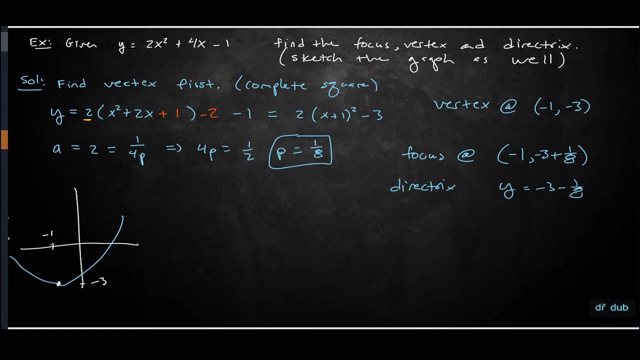 Well, if we look at the graph, our vertex is at negative 1, negative 3, it's down here And it's opening up because coefficient is positive. then our parabola is going to look like this. So I know my focus has got to be above that and my directrix has got to be below that. 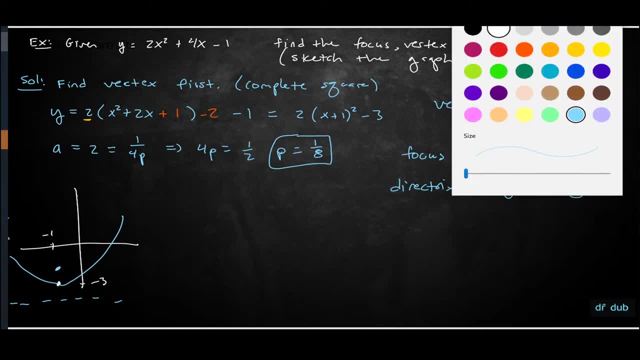 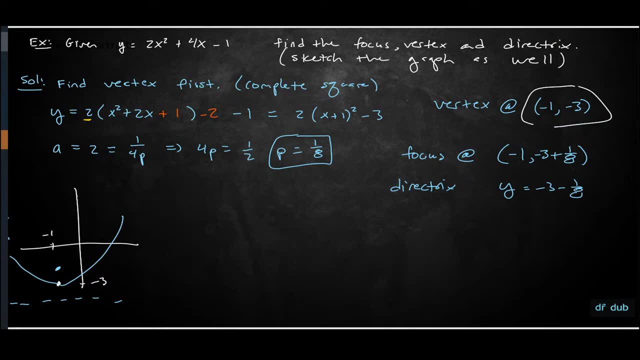 vertex. So that's how we can say what the focus in the directrix is. So I got the vertex right here. Let me just simplify. The focus is going to be negative 1 and then that would be negative 24 plus 1 would be. 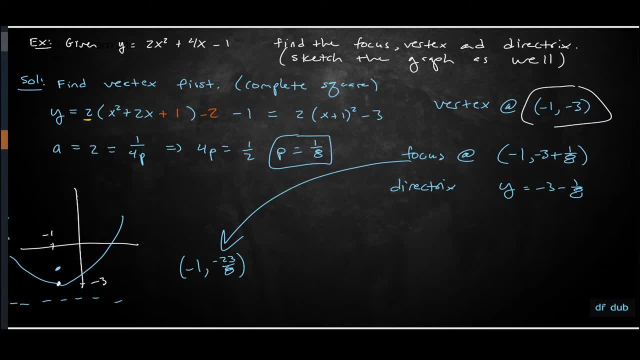 negative 23 over 8, that would be my focus And the directrix is going to be: y equals negative 3, let's see minus, so negative 24, so negative 25 over 8 would be my directrix. 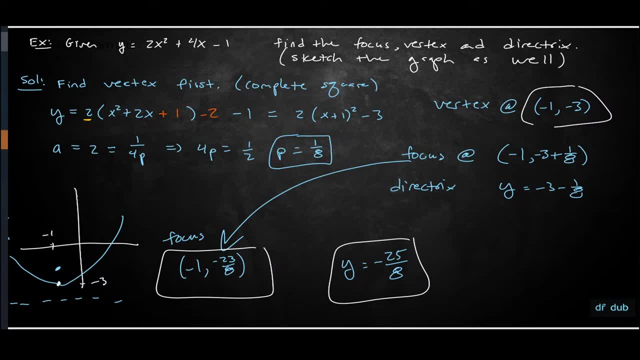 And the contract. So I'm going to have to add that to the present value. So the target is going to be negative 0, positive 0, negative 4, negative 5, negative 5 over 8.. And the directrix is going to be negative 4 over 8.. 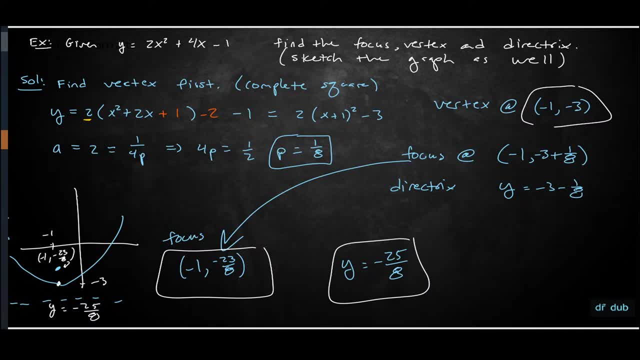 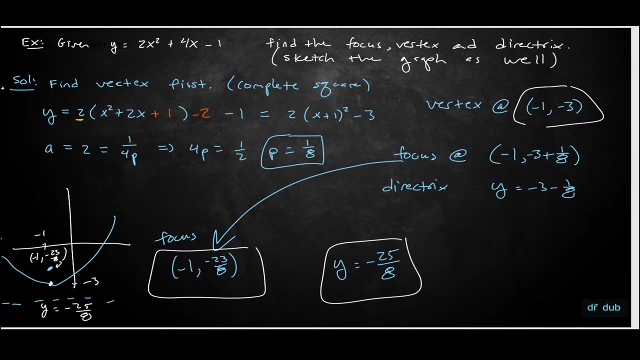 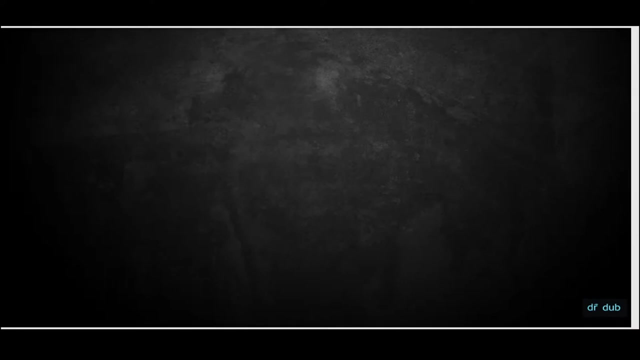 So I'm going to add that value to the present value, So I'm going to call this dx you, you. okay, if no questions, we'll move on to ellipses, ellipses, and again we'll look at the geometric definition. i won't derive the equation here, but we'll just 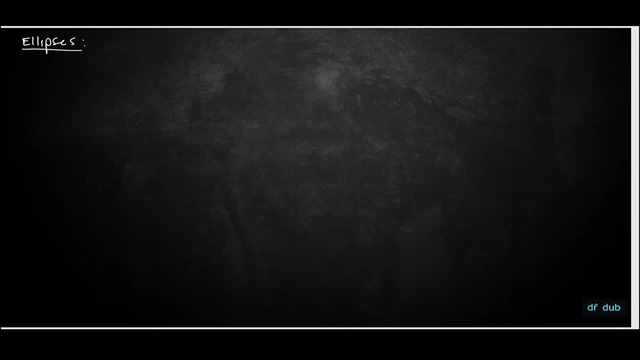 talk about the things that define an ellipse. so definition: an ellipse is the set of all points in a plane for which the sum of the distances to two foci is constant. so what does that mean? well, that means if you have an ellipse, then there are two things called foci. 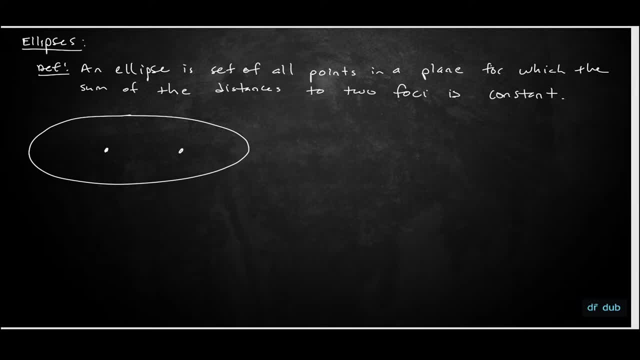 such that the distance to any point on the ellipse x, y, d1 and d2, D1 plus D2, is the same, no matter which point we choose on the ellipse. So that sum is fixed or constant, no matter what point we pick on the ellipse. 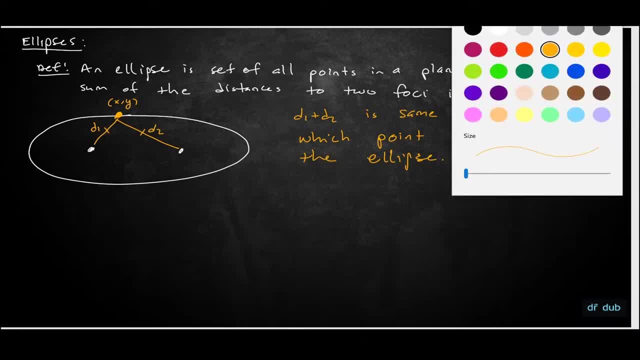 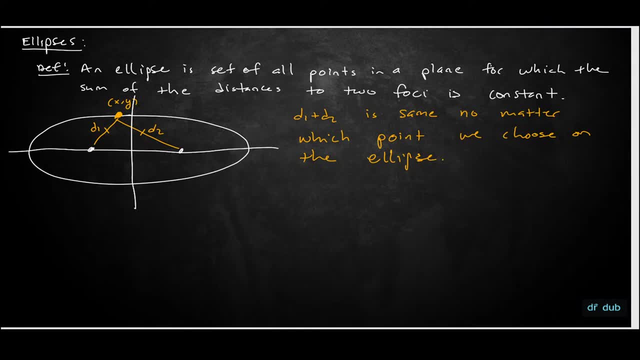 So I'm going to just finish the graph here a little bit. I'm just going to give you the unshifted graph. Okay, And call this vertex A0.. Call this vertex negative A0. This vertex is going to be 0, negative B. And then this vertex is going to be 0, B. 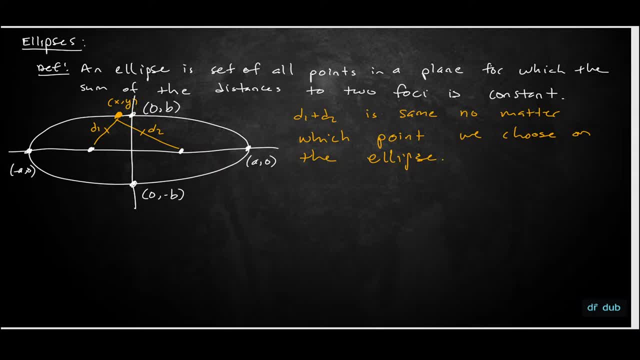 And this distance here is going to be C, Same thing here. So then, the unshifted ellipse equation- I'm not going to derive it, but the unshifted ellipse equation is: x squared over a squared plus y squared over b squared, equals 1.. 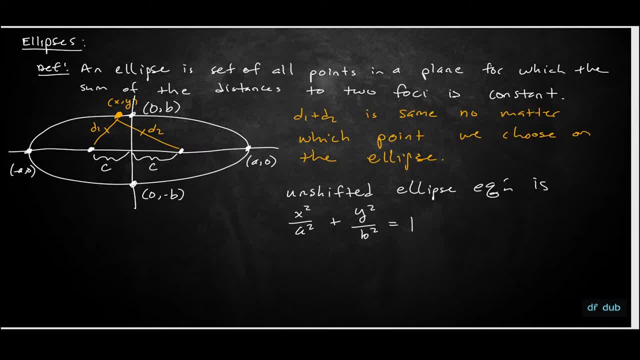 So that's the unshifted ellipse, Okay, Okay, Okay. So that's the unshifted ellipse equation, And from there we can shift it left right up down by changing x. You know, say x minus h, quantity squared, if you want to shift it to the right, by h units. 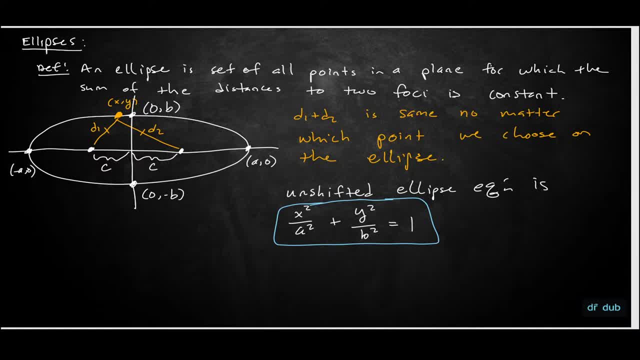 And you could do y minus k, quantity squared, if you want to shift it up or down- by k units, And then the foci are calculated. So the foci are calculated, Okay, Okay, Okay, It's going to be. n by c squared equals a squared minus b squared if a is greater than b. 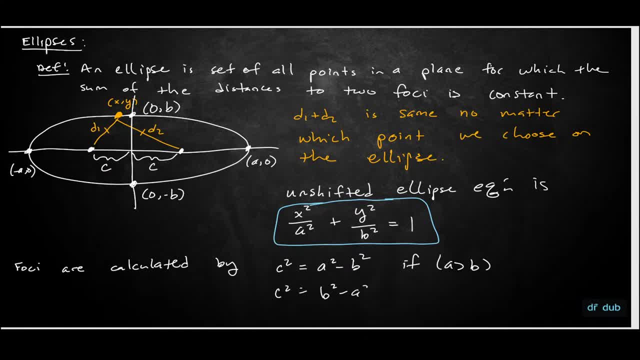 And c squared equals b squared minus a squared if b is greater than a. So depending on which one's larger, that tells you how it's elongated. Okay, denominator of x is larger, then it's longer in the x direction. If the 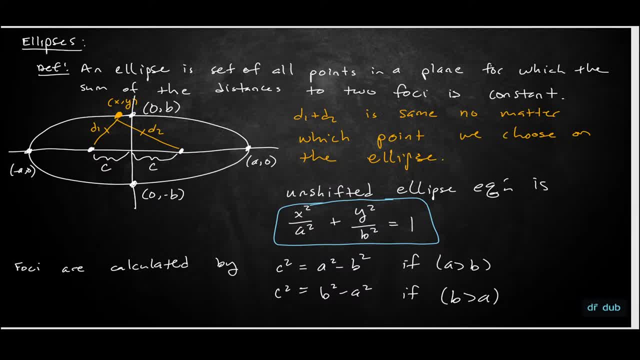 denominator of y is larger, then it's longer in the y direction. If the denominators of x and y are the same, it's just a circle. So depending on which axis is longer, we call that the major axis. So the major axis is the longer. 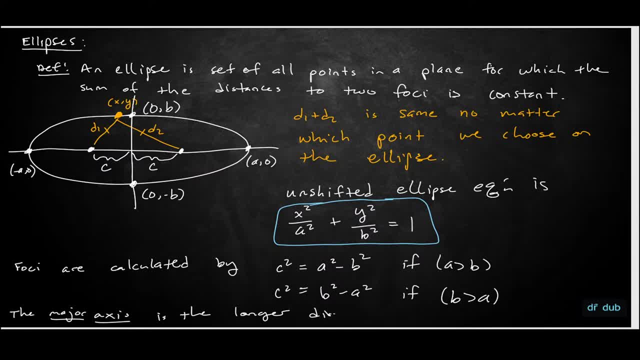 direction. So if b is longer, then it's the y direction, And if a is longer or larger, then it's the x direction, the major axis, or the major axis. So in this case, because I elongated it in the x direction, the major diameter. 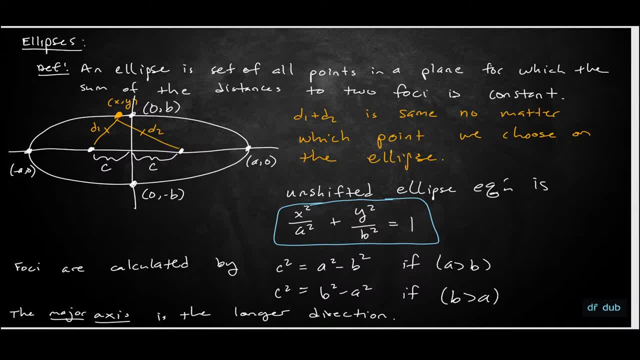 would be 2 times a, So in this the major diameter is 2a, the way I've drawn the ellipse here, And then those would be your foci, depending on which axis is longer or which where the elongation takes place. 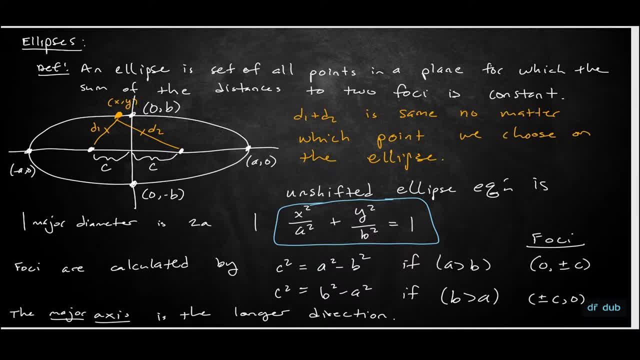 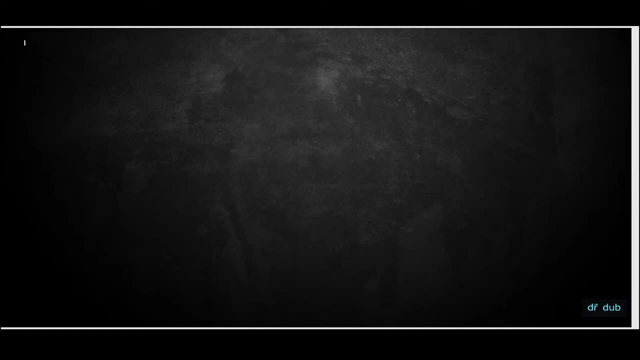 Okay, We've got an example. So the example says that 13x squared plus 2x plus y squared equals 1, represents a shifted ellipse. So we're going to take the ellipse, find its center point and the length of the major. 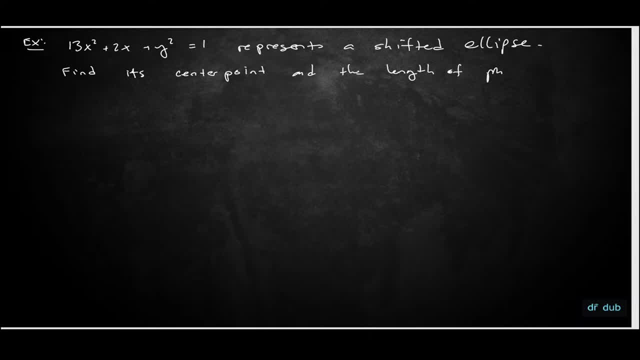 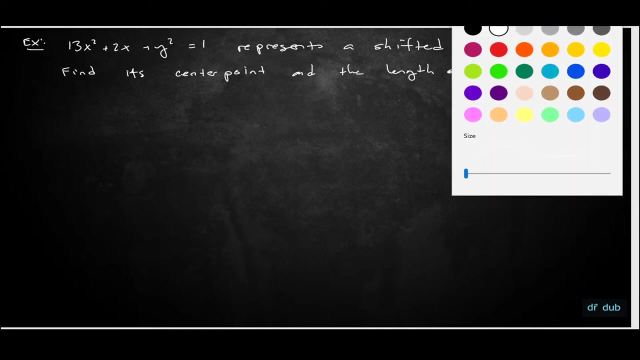 axis. So we're going to take the ellipse, find its center point and the length of the major diameter. So I want to find the center of the ellipse. That shouldn't be too hard. Just complete the square But then find the major diameter. 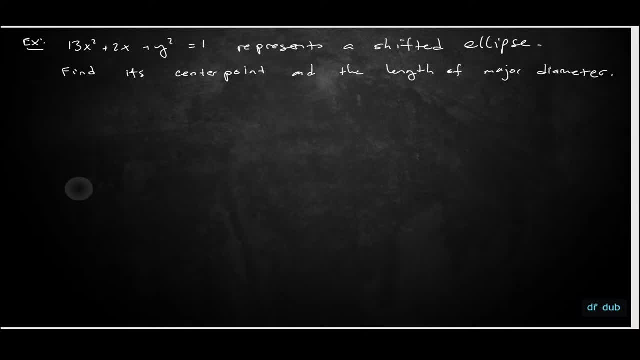 That is going to be a little bit work conceptually. So complete the square, So complete squares is the first thing we do. So I'm going to say 13 and then x squared plus 2 over 13x plus, then something we don't. 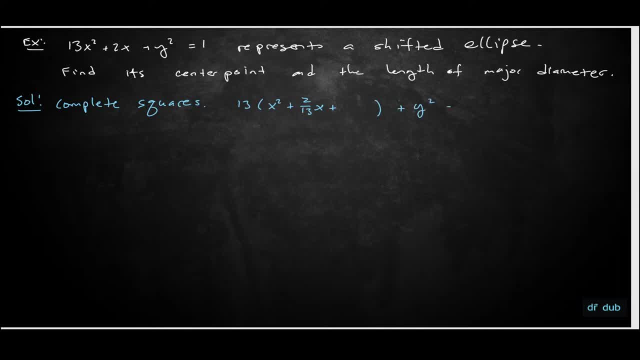 know, plus y squared equals 1.. And now I have to add something. So I'm adding to both sides. And what am I going to add to both sides? Well, I take 2 over 13 and get 1 over 13, and then square that to get 1 over 169.. 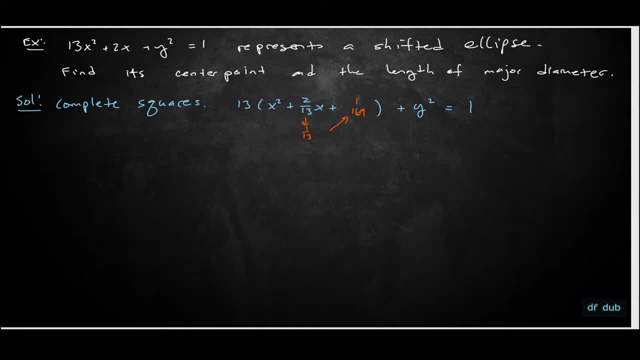 So I'm adding that to both sides, but actually it's being multiplied by 13.. So actually I add 13 over 169, which is just 1 over 13 to both sides. The y is already complete. I don't want to add anything. 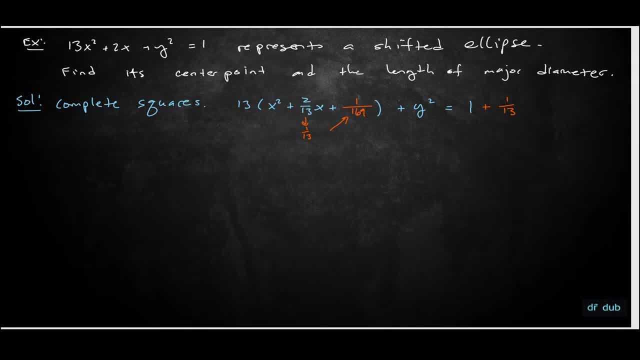 I don't have to complete the square there. So this is going to give us 13 times x plus 1 over 13. quantity squared plus y squared equals 14 over 13.. So the square is complete. but this isn't really the form of the ellipse. 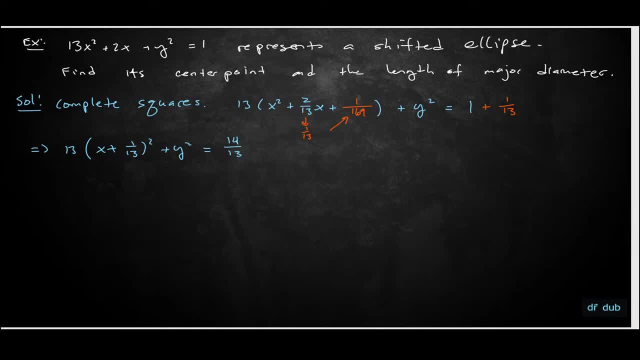 I need a 1 on the right-hand side. So multiply both sides by 13 over 14.. So multiply both sides by 13 over 14. And that's going to give us 169 over 14 times x plus 1 over 13, squared plus 13 over 14y. 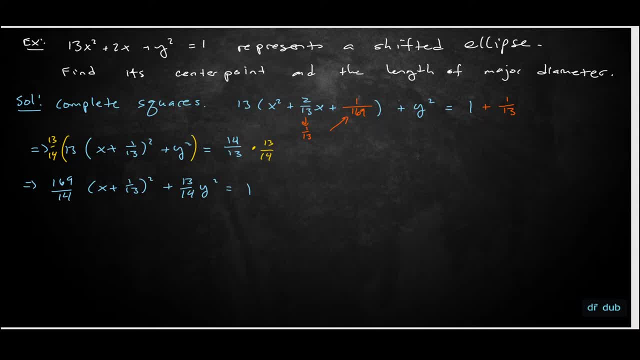 squared Equals 1.. So almost there I've got a 1 on the right-hand side. but on the left I have coefficients in the numerator. I actually need them to be in the denominator. So how do I make those fractions in the numerator move to the denominator. 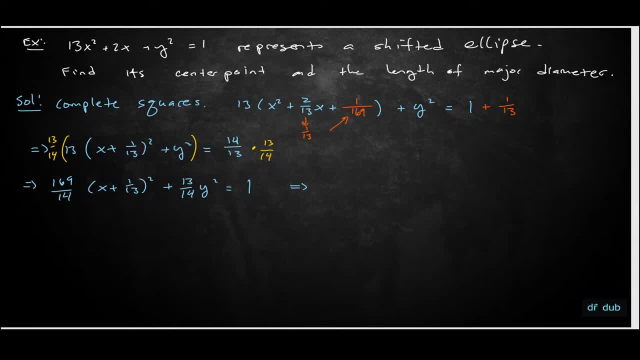 Well, I just need to take the reciprocal and put them in the denominator. So this is going to be x plus 1 over 13, squared over 14.. 14 over 169 plus y, squared over 14 over 13, equals 1.. 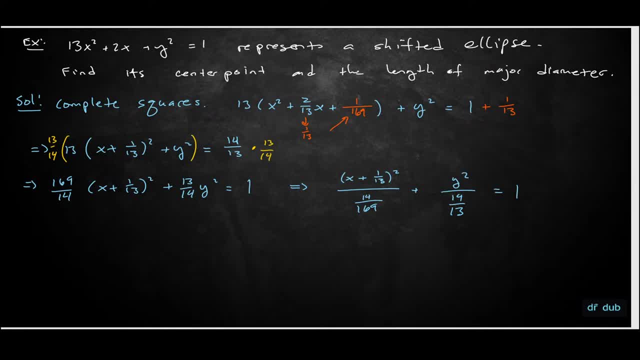 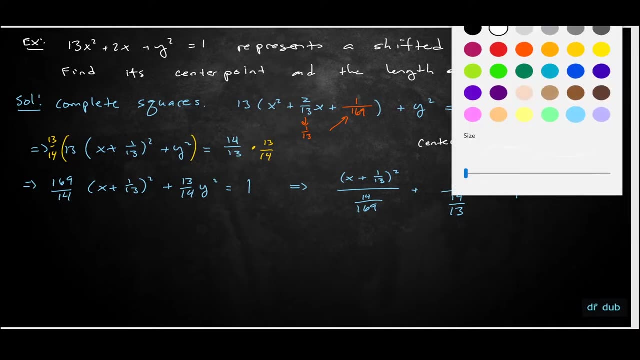 And I already can see the center point, of course. So the center point is going to be the point negative 1 over 13,. comma 0.. And which denominator is larger? Okay, So a squared is equal to 14 over 169.. 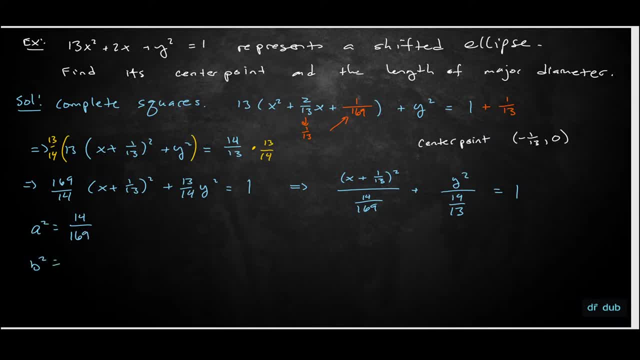 B squared is equal to 14 over 13.. So definitely a is less than b, So a is less than b. So this is elongated in the y direction. B is equal to square root of 14 over 13.. So then the major diameter is 2 times b, which is going to be 2 times square root of 14 over. 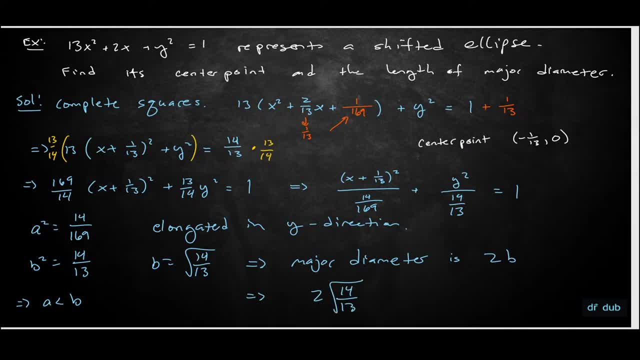 13. And that's our major diameter. B is equal to square root of 14 over 13,, comma 1 over 13,, comma 1 over 13,, comma 1 over 13.. Questions about that. 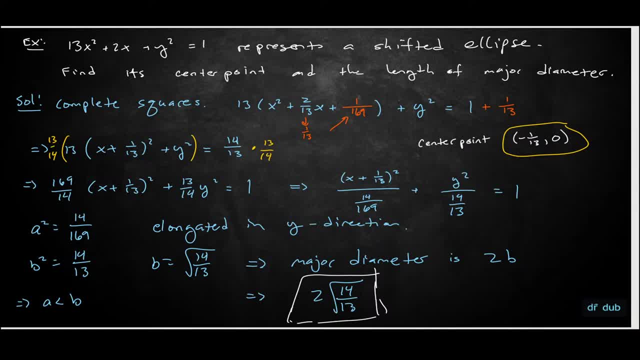 Cool, cool, Cool cool. So just kind of understanding. you know the foci directrix, things like that. In this case it's just a foci center point, vertices, things like that and an ellipse. 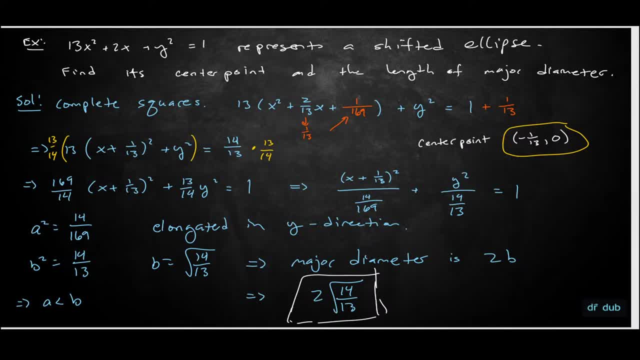 That's just the new stuff. I didn't tell you to calculate the foci here. I guess I could have. Would be pretty nasty because a and b are not very nice to work with. We could have calculated the foci. We could have calculated the foci using the formula at the bottom here. 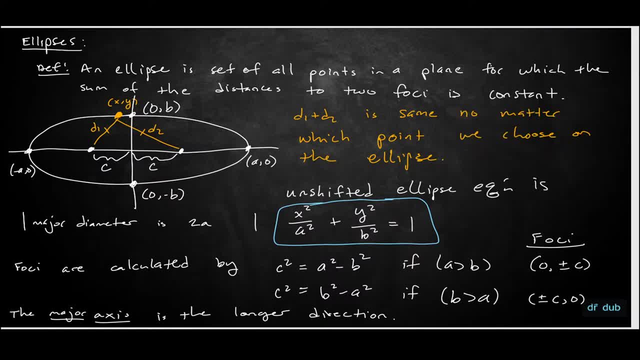 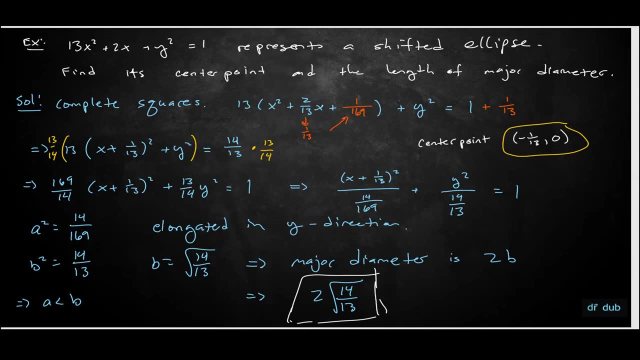 So foci we could have calculated using, let's see, b is larger than a, so we would have used this formula And then the foci would have been here. But the problem didn't say to do that, so we're not going to worry about that. 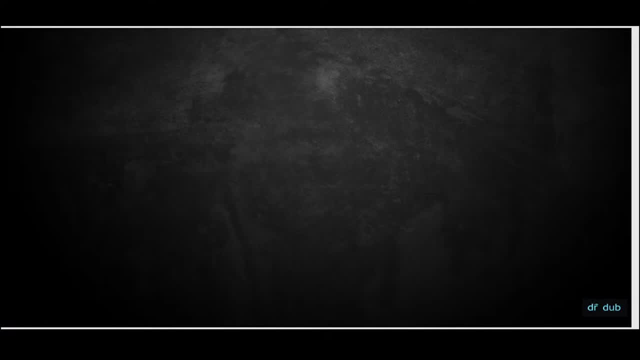 Let's look at the log, Let's look at the last conic section, and that is a hyperbola. So hyperbolas, So hyperbolas, And they're actually just like they're almost exactly the same as an ellipse, except instead of taking the sum and making that a constant. 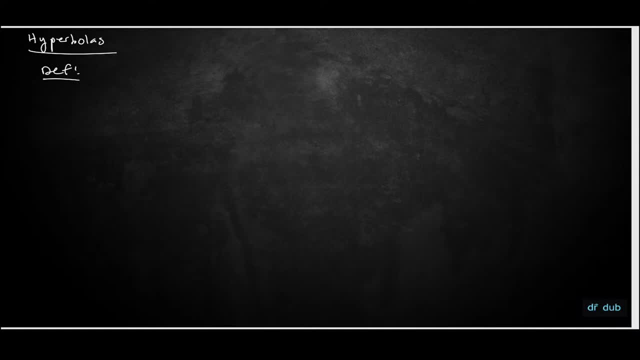 we make the difference. The distance is to two points the same, So it's like an inverted ellipse, almost. So. the geometric definition is a hyperbola, is the set of all points for which the difference of the distances to two foci, oops. 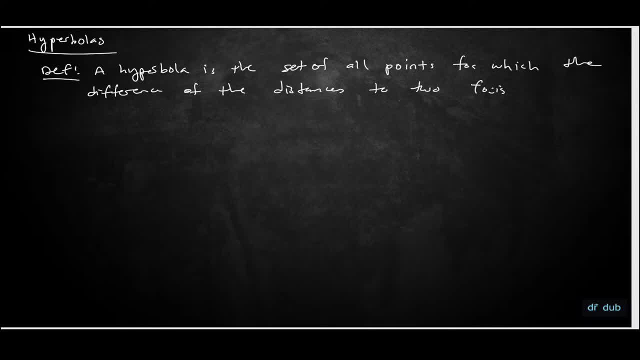 to foci. oops, to foci is constant, So it's very similar to an ellipse, except we say difference instead of sum, and that changes everything. So let's look at that. I have a focus right here and a focus right here. whoops, they kind of need to be on the 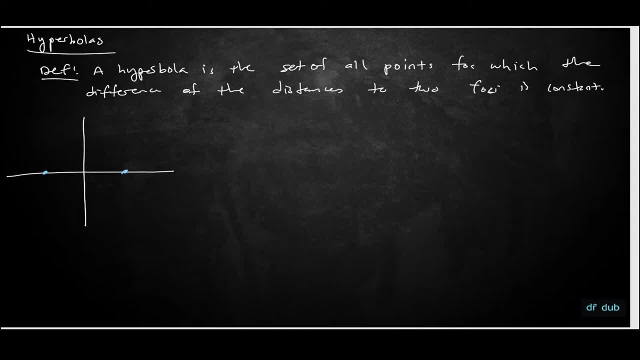 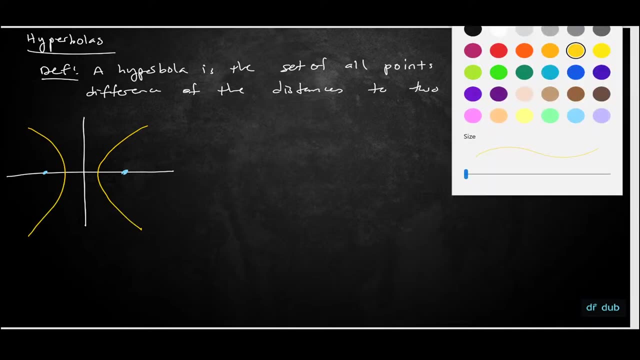 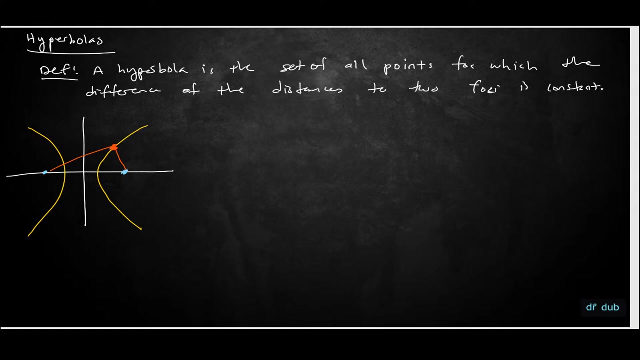 same distance scale right there, Then the hyperbola is going to look something like this: So the distances are here and here. so this is the point on the hyperbola, and we'll call this d1 and d2.. And that's our focus. 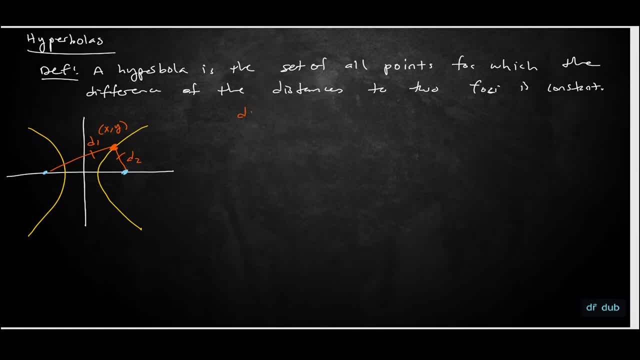 D2,, and so D1 minus D2 is fixed for every point on the right branch, and D2 minus D1 is fixed for every point on the left branch. Of course we could rotate this and make it a vertical hyperbola, and then we have a top. 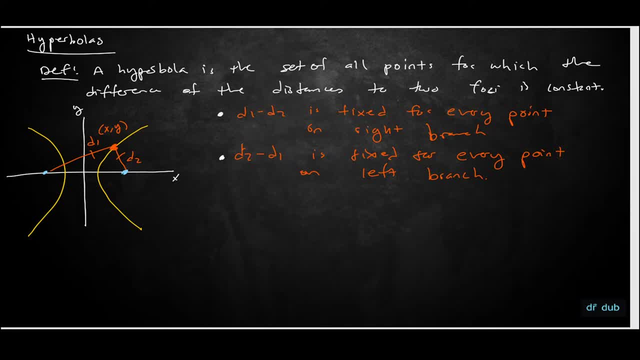 branch and a bottom branch, and we'll talk about that in just a second. So the equation of this hyperbola would be: x squared over a, squared minus y, squared over b, squared equals 1, and we have two vertices right here. This is x equals a and this is x equals negative a. but we don't have any y vertices because 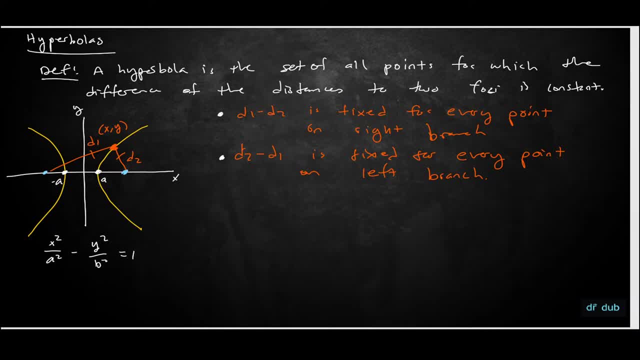 if we set x equal to 0, we get an imaginary number for y, so there are no vertices in the y direction And c squared is equal to a squared plus b squared, and c is where the foci are. so c and negative c. 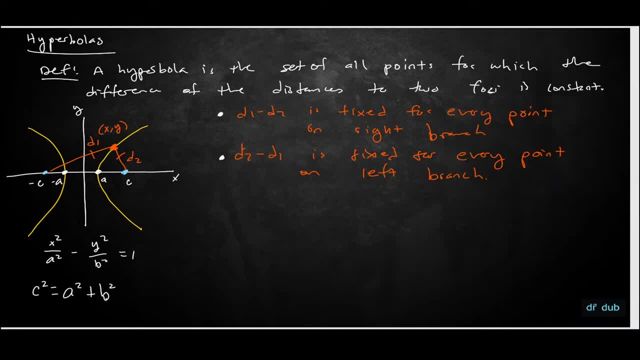 And in the hyperbola there are two vertices, There are two asymptotes that the branches will never cross and if you have a left branch, right branch situation, the asymptotes are the one over here. on the left is y equals negative b over a times x. 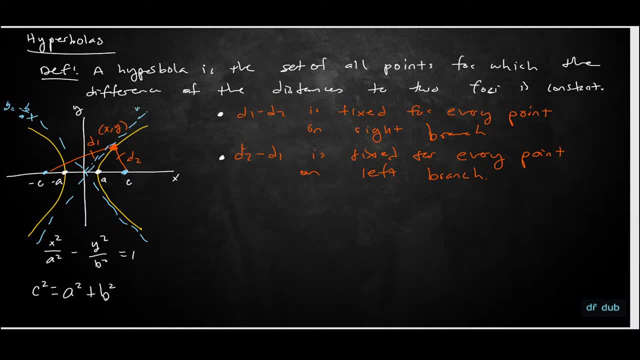 And the one on the right is: y equals a squared over b squared over a squared over b squared, y equals positive B over a times X. so that's the unshifted hyperbola. forget the up-down hyperbola, very similar. so you got to foci again and the branches. 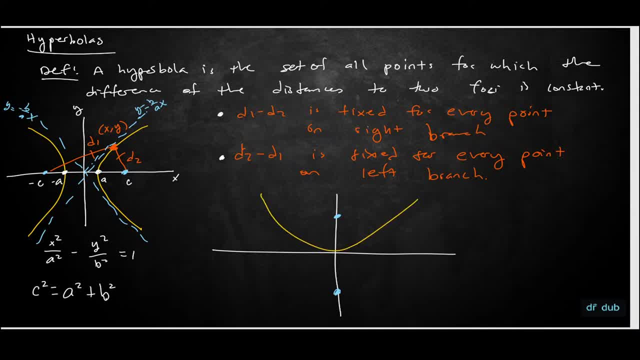 would be something like this: well, maybe not touching the origin, not very good. you to parabola like: there we go, it's too pointy. there we go, that's pretty good. maybe a little close, but oh well, let me just move this focus down a little bit. 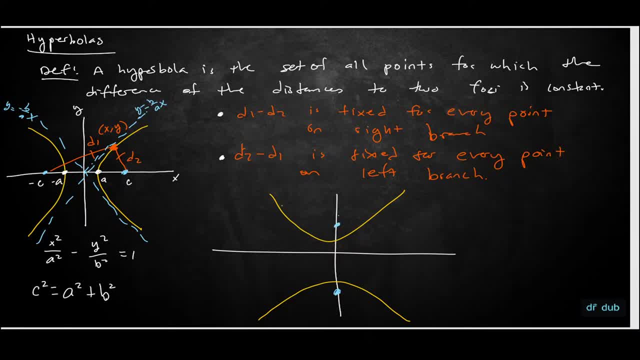 okay, if you have a parabola or, sorry, a hyperbola looks like this, then the equation is: Y squared over B squared. okay, if you have a parabola or, sorry, a hyperbola looks like this, then the equation is: Y squared over B squared, minus X squared over a squared equals one and C. 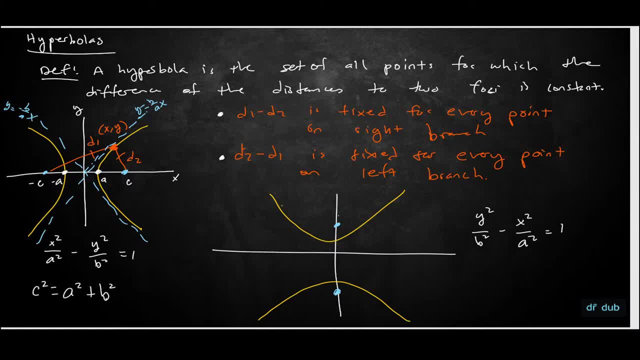 squared is still the same thing. so C squared is equal to a squared plus B squared in both cases. but now we have vertices: at Y equals B and Y equals negative B. okay, at C and negative C. but then also we have asymptotes again, but now it's Y. 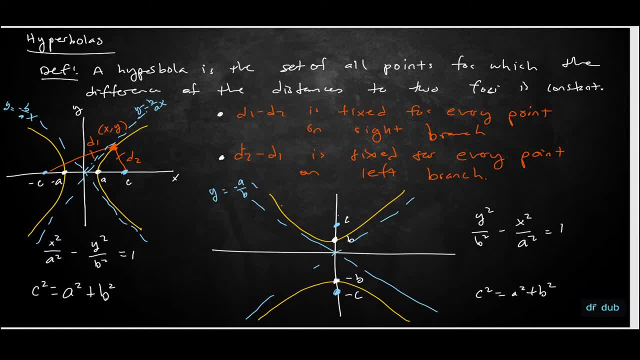 equals negative a over B over here, and then Y equals negative positive a over B times X up here. so those would be the unshifted hyperbolas и casi. again, I'm not gonna derive these these here, but I think the derivations in the book if you really really want to look. 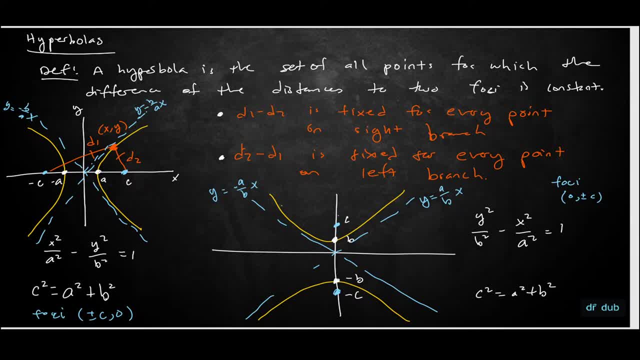 at it here. so you're gonna work with any of these derivatives of your choice. I'm gonna pass my assets to the 건데 RA and we'll do. now is another example, so it'll be. Let's look at an example. see if there are any questions. first, 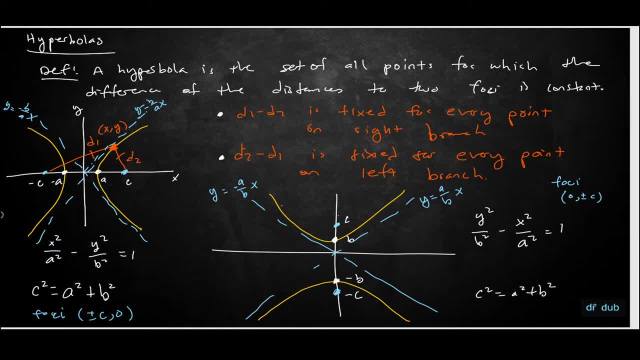 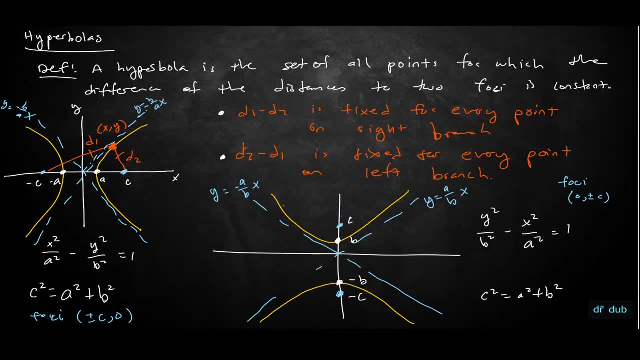 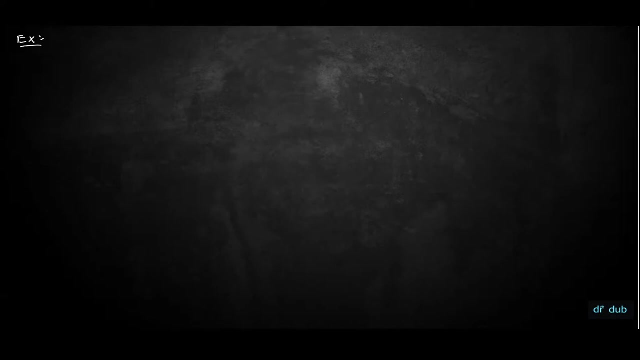 Okay, if there are no questions, I guess we'll just look at an example and then finish up our discussion with a more general form for these conic sections. So one example we can do here. it's pretty straightforward, actually just says: find 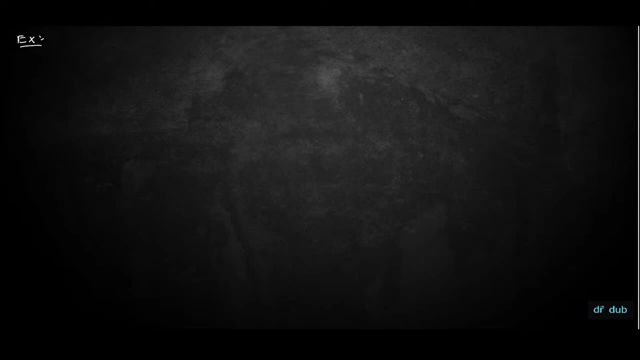 the vertices, foci and asymptotes. For example, find vertices, foci and asymptotes of x. So y squared over 16 minus x squared over 36 equals 1,. okay solution. So we have a squared is 16, we have b squared, which is 36.. 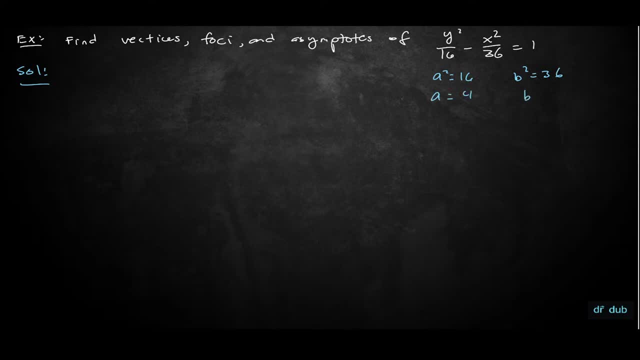 And so we can automatically get a squared over 16 minus x, squared over 36, equals 1.. So we have a squared over 16 minus x, squared over 36, equals 1.. So we have a squared over 16 minus x, squared over 32, which is 4, b, which is 6.. 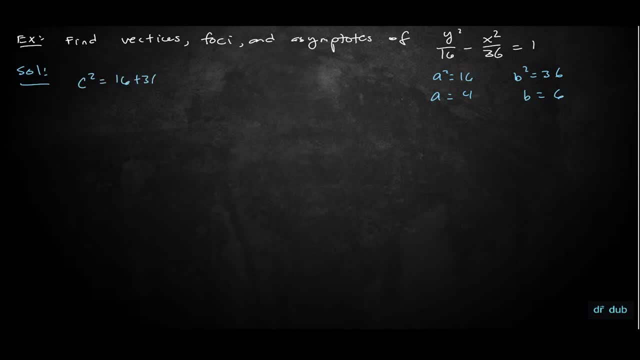 And also c squared is going to be 16 plus 36,, which is going to be 52.. And so c is going to be square root of 52,, which we could say is 2 square root of 13.. And so the vertices, let's see which one's larger. 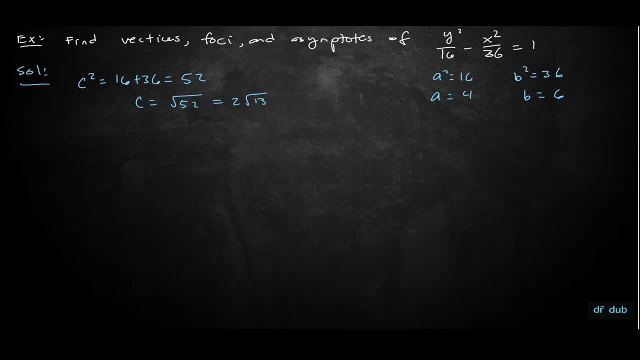 Well, yes, it doesn't matter. The y is first and the negative is in the x direction. So we have a vertical hyperbola. So our vertices are at b and negative b because this thing's unshifted. So our 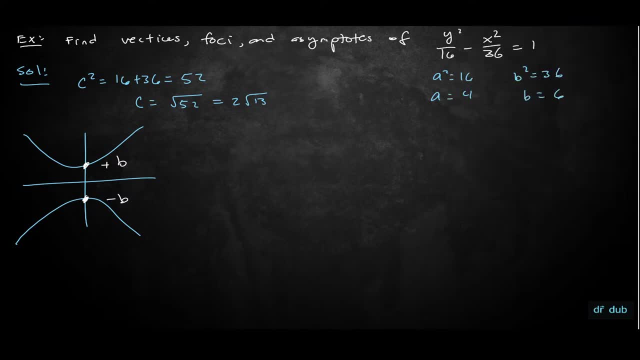 vertices are going to be at zero plus minus six, And the foci are going to be at zero plus minus two square roots of 13.. And then our asymptotes are going to be: y equals plus minus a over b times x, which is going to be plus minus four over six times x, which is y equals plus. 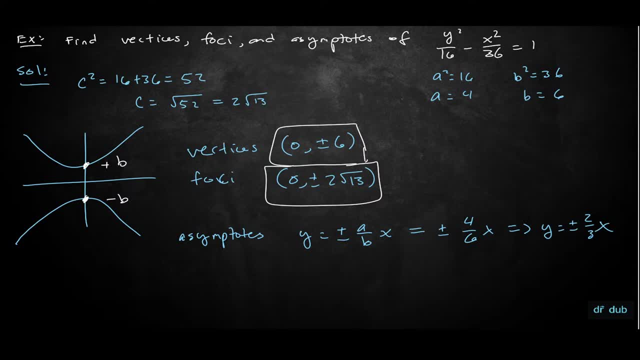 minus two over three x, And that is it. Any questions? Okay, cool, We will look at a general form of conic sections and kind of determine if we know how it's going to be an ellipse, parabola, hyperbola. 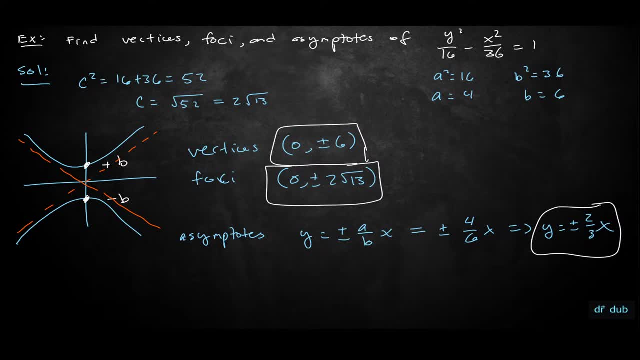 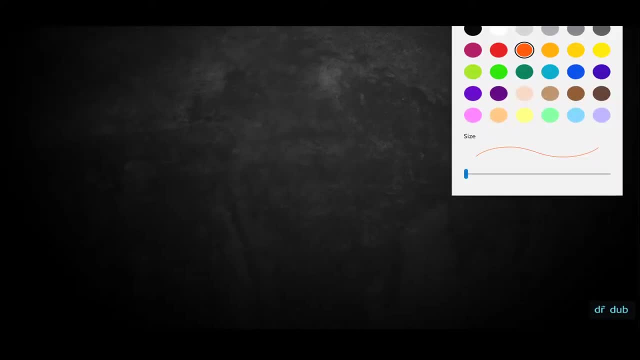 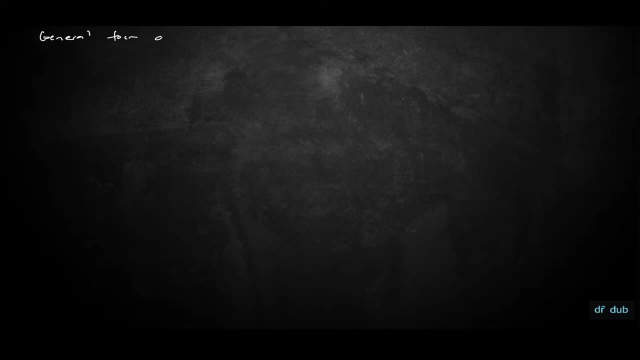 From that and then look at the general shifted equations for each one. So let's look at the general form of conic sections. So the general form of conic sections, And that is ax squared plus bxy plus cy squared plus dx plus ey plus f, equals zero. 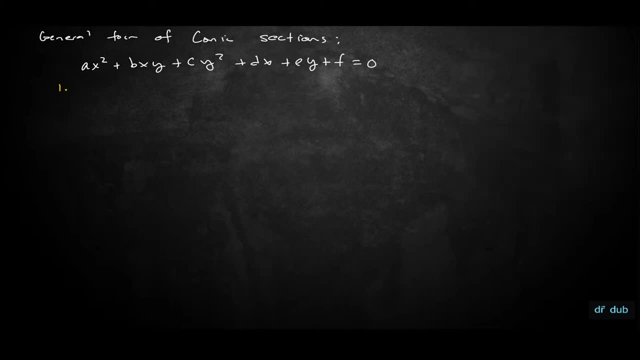 And there are three conic sections. we know One, two, three. And how do we know? So? if b squared minus 4ac is greater than zero, 0, then hyperbola. If b squared minus 4ac equals 0, then it's going to be a parabola. 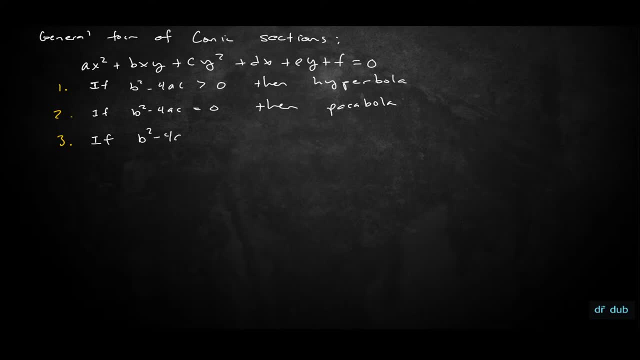 And if b squared minus 4ac is less than 0, then it will be an ellipse. And this general form of the conic section is any rotated hyperbola, Any type of weird stretching things like that, So shifting. it's all captured in this general conic section equation. 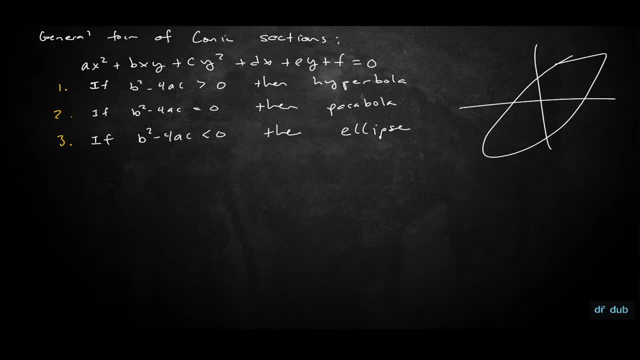 So you could have an ellipse that is rotated, something like this with this general form of the conic section. So something like that is covered right here. So if you look at the general shifted forms of conic sections or the equations, so the general 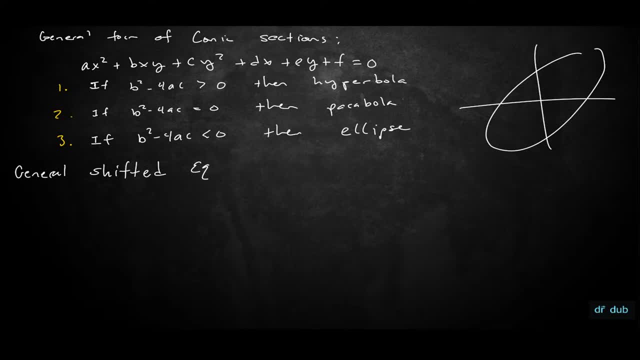 shifted form of conic sections or the equations. number one could look at a circle which is x minus h squared, plus y minus k squared equals r squared, and that's a circle. Could have an ellipse: x minus h squared over a squared. well, I should use a different letter. 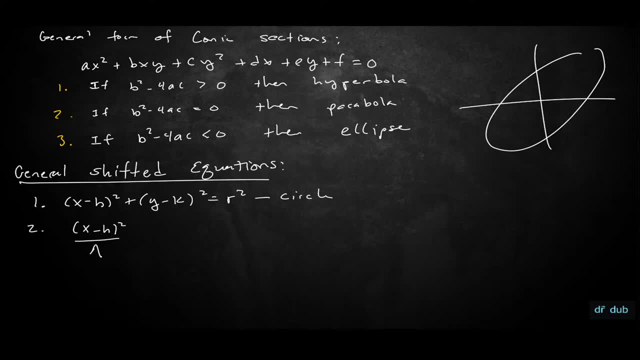 because I have lower case a already call it capital. A squared plus y minus k, squared over b squared equals one, and that's a ellipse. Number three could have hyperbola: x minus h squared over a squared plus y minus k, or actually minus y minus k squared over b squared equals 3, along with u squared. Let's update this for the turtles. Remember, only a look will do So. this is really painful because we need a time to enjoy this chart And, of course, I want to give you an update if you have any questions. Anyway, if you have any questions, just leave a comment below. 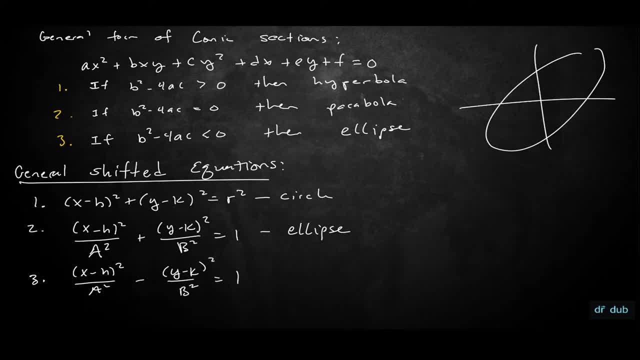 Ease of thinking. for hours I'll beseeing you guys at the end. I'll bebishing the call too soon. Bye, bye, Thank you, Thanks. 이런 bye, bye You too, equals one, that's. uh, that would be a left right hyperbola, so left right hyperbola. 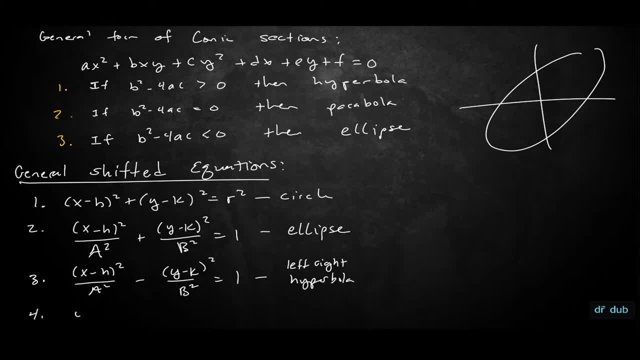 and then number four. we could have a parabola which would be something like: y minus k equals one over four, p times x minus h squared, and that would be an up down parabola, up or down parabola. so just to give you an idea of the general. 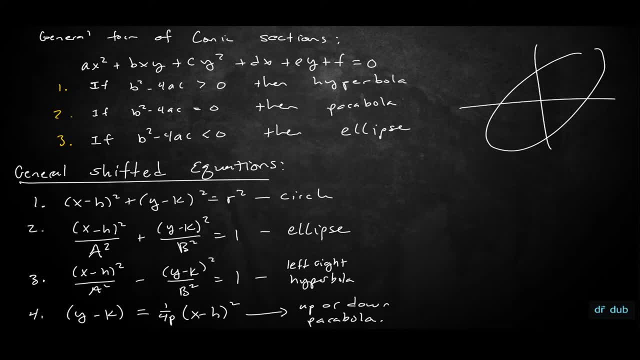 shifted equation what they could look like. so that would be shifted up by k units and right by h units for that parabola. so the vertex would be h k, focus would be h plus or h k plus p, and directrix by equals: k minus p. 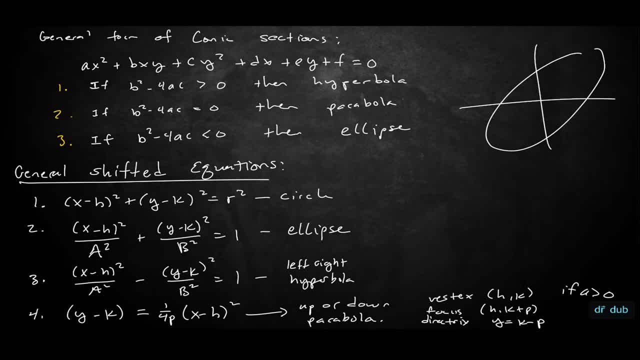 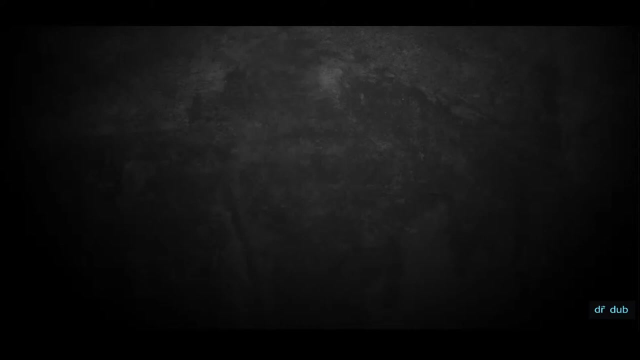 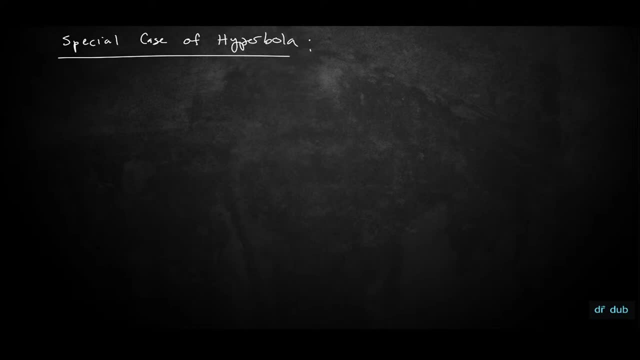 a circle is a special case of an ellipse. there's a special case of a hyperbola I want to focus on, and that's the special case x-axis. x-squared over a-squared minus y-squared over b-squared equals zero. and so then you 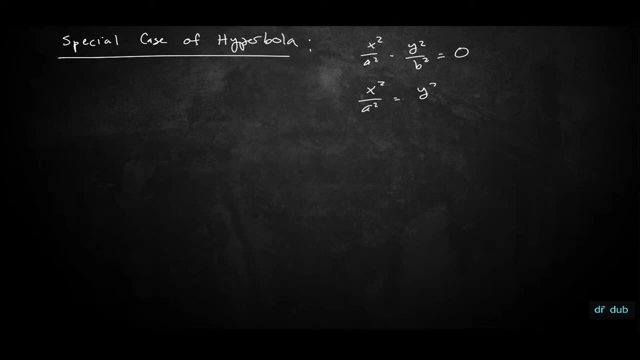 would have: x-squared over a-squared equals y-squared over b-squared, and so you could say: y is equal to plus or minus b over a times x, and then it's just two intersecting lines. so it's just two intersecting lines. 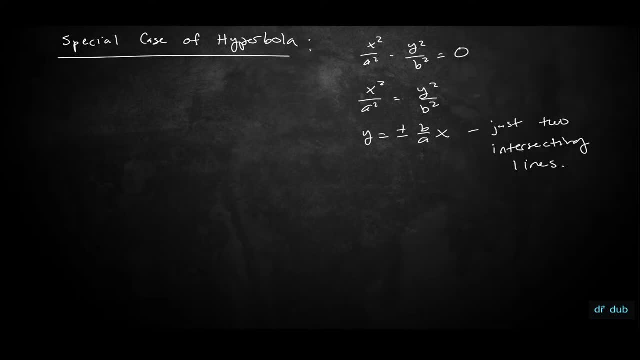 Basically, if you get a zero, Okay, On the right hand side, you're going to end up with two intersecting lines. If you complete the square and you get a zero on the right, it's just two intersecting lines. So it's basically just the two asymptotes. 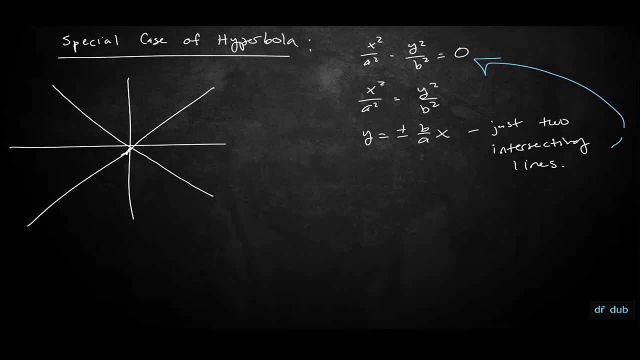 Okay, So the defined number is the order of your asymptotes down to x's, and then the squared computer is the stopping point and theiam number two is the end of your stitches. Beautifully done, Okay. Transノ, graceful demais. 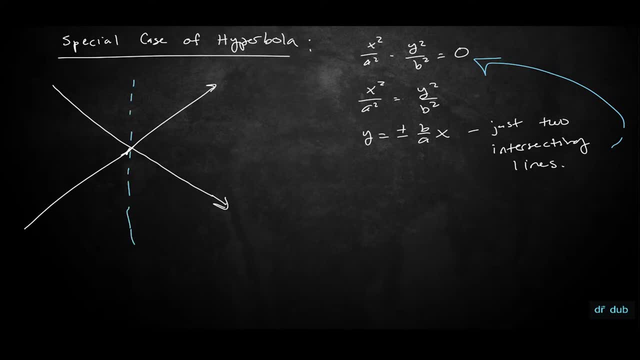 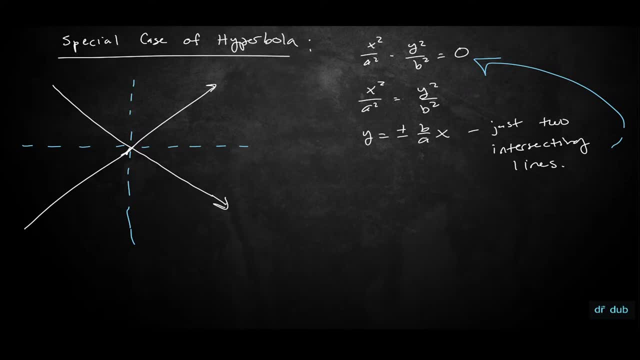